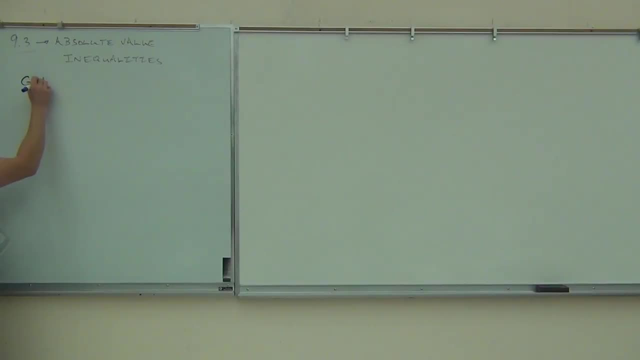 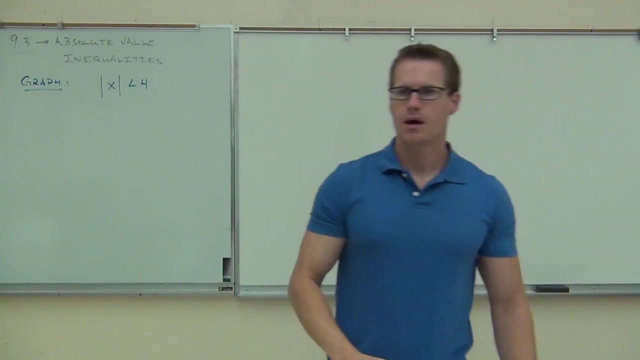 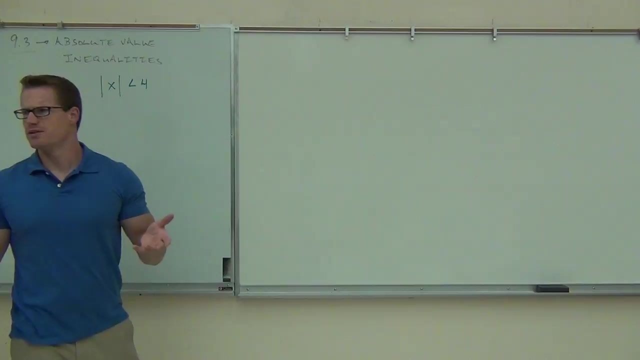 So let's go ahead and let's graph, And I'll explain- absolute value of x less than 4.. Now what I'd like to do. I want to start off by thinking about some of the numbers that are in this set. We all know what absolute value does, right. Absolute value makes anything that you put in there positive. 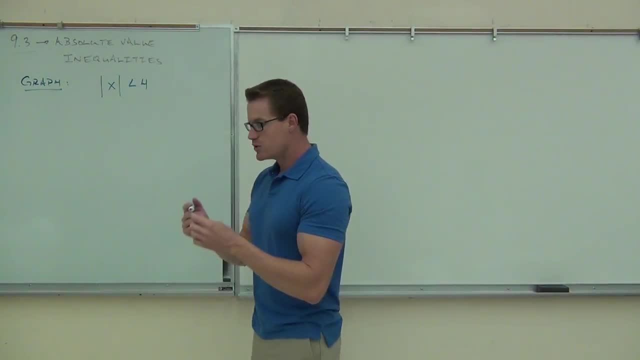 If it is positive, it remains positive. If it's negative, it becomes positive. Can you give me a number that satisfies this expression, this inequality, 1.. 1 satisfies it. Great 1, absolute value of 1 is 1.. Is that less than 4?? 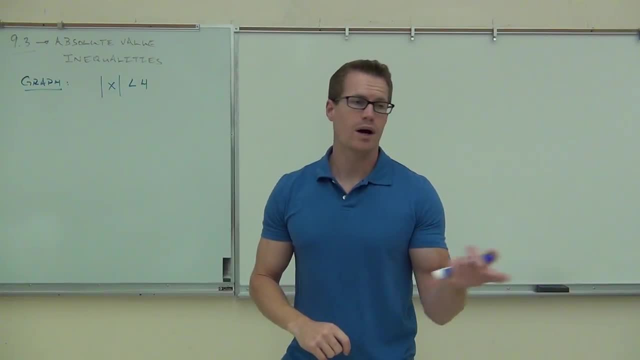 Yeah, Give me another one. Negative 2., Negative 2. Why negative 2?? It's still less than 4.. Sure, Okay, How about what else? Say that again? Negative 4., Negative 4.. How about negative 4?? 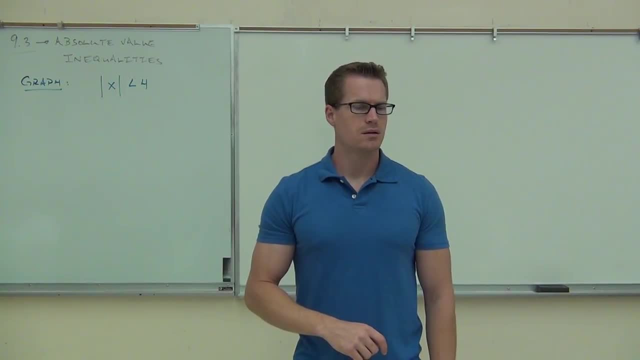 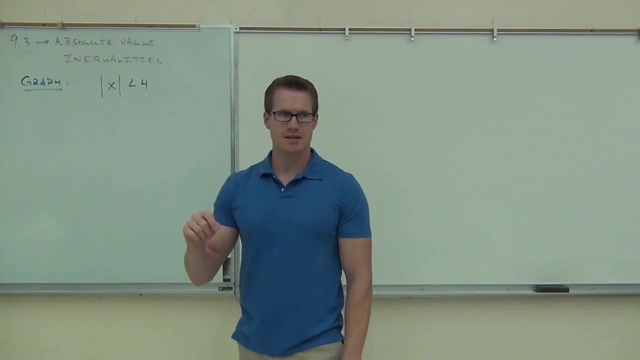 No, Well, why not? Because it's going to turn positive. Oh so if I put in negative 4, absolute value of negative 4 is 4.. Is 4 strictly less than 4? No, No, So that would not work. Give me another one that does work. 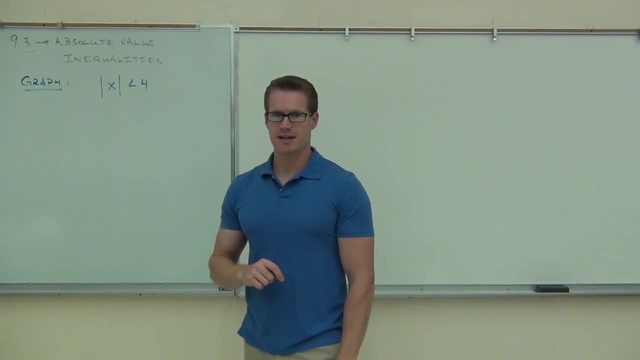 3.9999.. Negative, Negative, Negative: 3.9999999999 forever. Absolute value of negative: 3.9999999999.. That's supposed to be 999.. Forever is positive: 3.99999999 forever. Is that less than 4?? 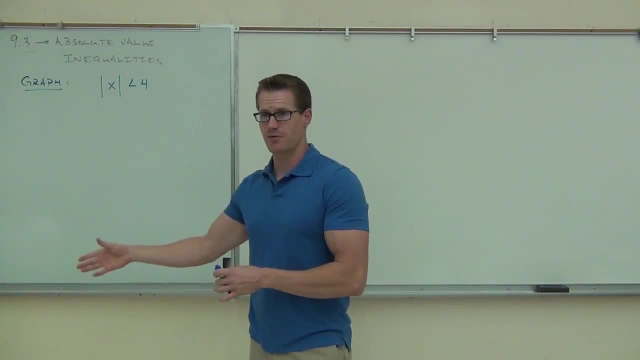 Yes, Then yes, that would work. 3.999999, forever. would work, because absolute value of that is still positive. How about 4?? Would 4 work? No, No, because absolute value of 4 is 4.. That is not less than 4.. How many people understand what these numbers look like? 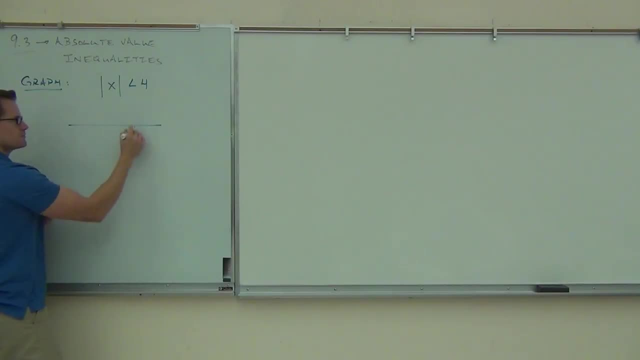 So if we were to do this on a number line, I can't plug anything in greater than 4.. Because that seriously would be greater than 4, right, in absolute value, Here's 0.. But I also can't plug anything less than negative 4.. 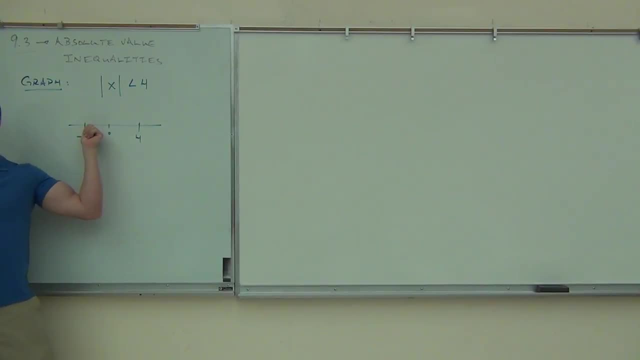 The reason is, if I plug in anything less than or equal to negative 4 in absolute value, that changes it to a positive, which then becomes bigger than 4.. Are you with me on this, ladies and gentlemen? So when I graph this, what this is is I'm going to use parentheses to signify that this is open. 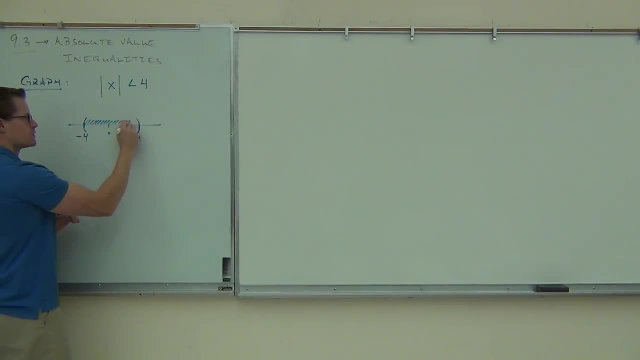 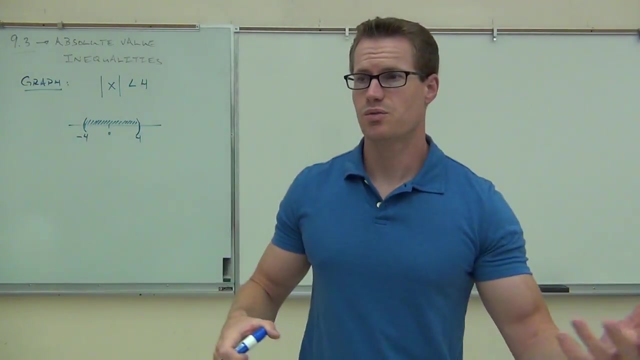 What we're talking about is this range of numbers in here, Anything between negative 4 and 4,, but not inclusive. The reason why it's not inclusive is why? Why is it not inclusive? Yeah, there's no equal sign up there. Very good. 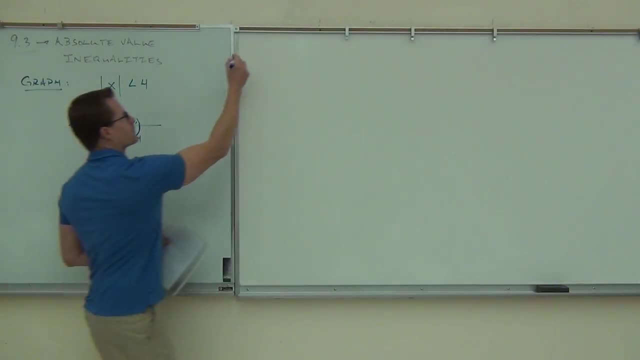 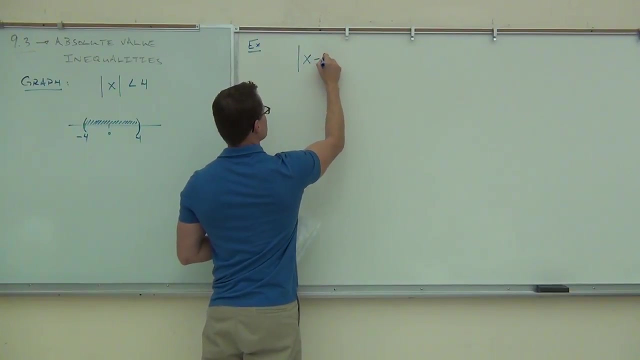 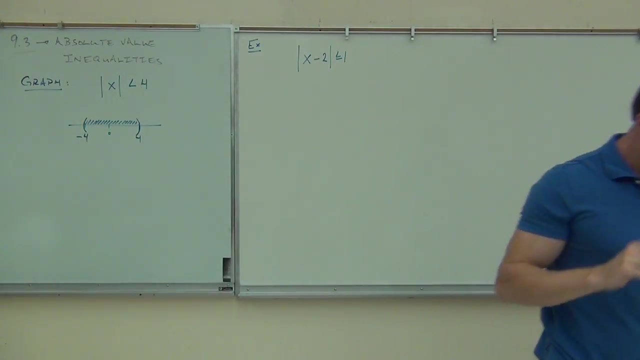 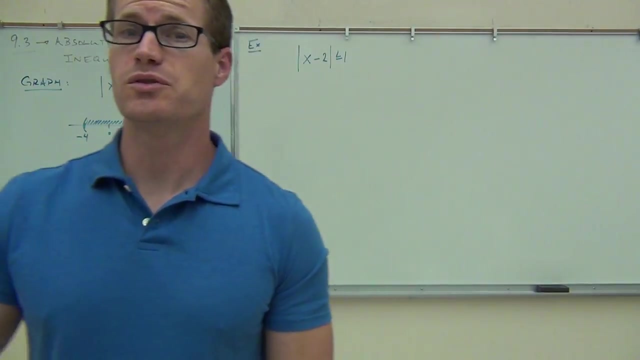 Let's see if we can take this and run with it. Hey, when we first started dealing with absolute value, how many equations did you get with absolute value? No matter what, you get 2, right, Hopefully. in your homework you got 2 in every single case. 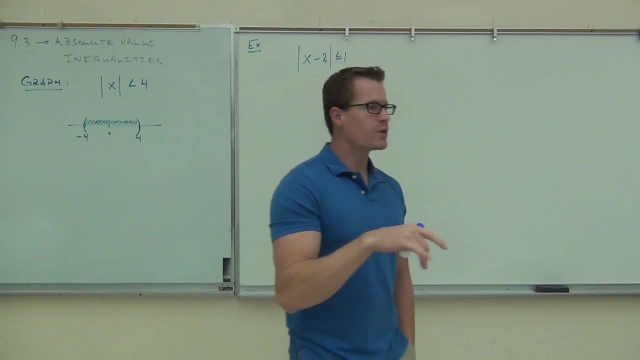 I hope you did that. You're supposed to get 2 in every single case. Well, if we get 2 equations when we're dealing with equations or absolute value equations, then when we're dealing with absolute value inequalities, we should get how many inequalities do you think? 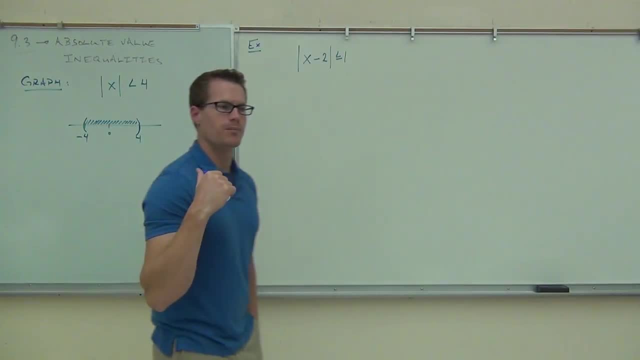 2.. As a matter of fact, I want you to look over here at this problem. When we did this problem, notice how we could have actually written out 2 inequalities. We know 2 things about this. We know that, firstly, x had to be less than positive 4.. 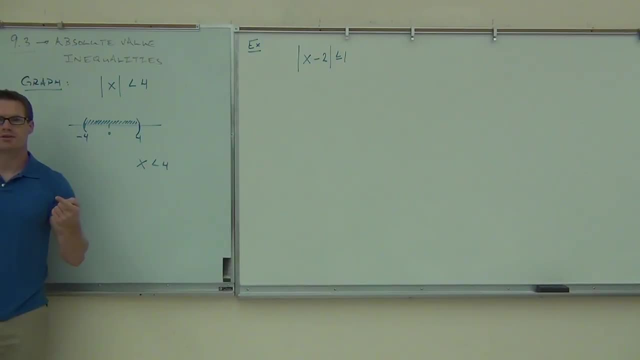 You with me on that. But we also knew another one. Check this out: x had to be greater than negative 4.. Didn't it? x had to be less than positive 4,. x had to be greater than negative 4.. 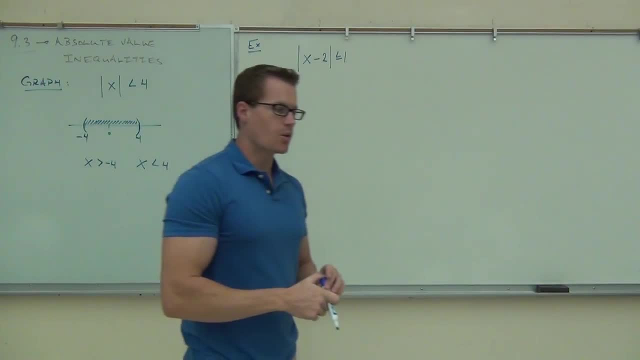 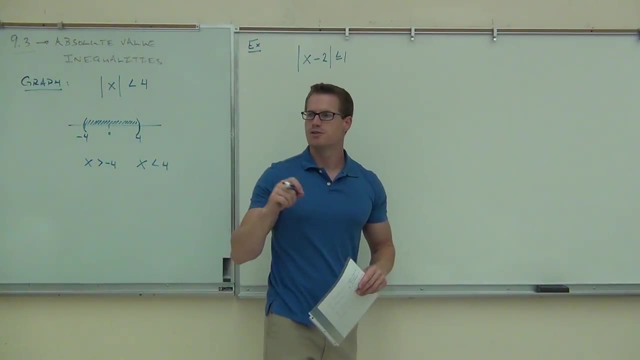 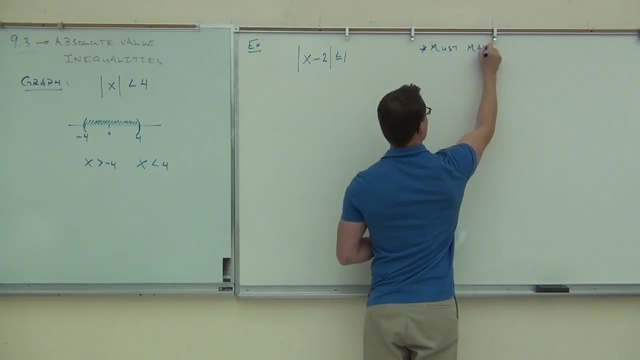 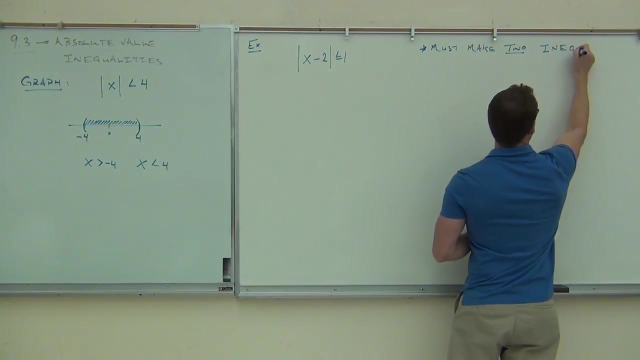 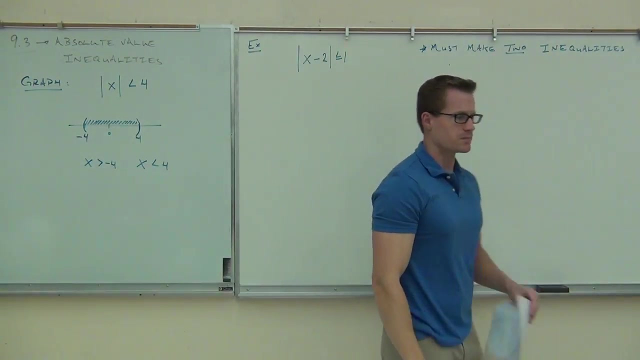 We actually make up 2 inequalities. So when we do this absolute value, inequality stuff, it is an absolute value, so we will have 2 inequalities. Let's do it again. Okay, how do we do it? Look back over here at this first example: okay. 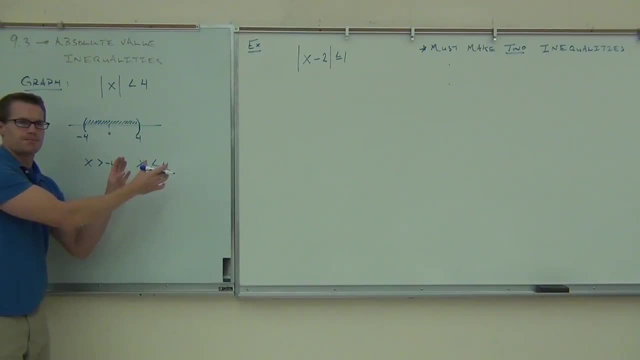 When we make up our 2 inequalities. look what happens. Look, Do you see that this one is really similar to the first absolute value? This is the first absolute value equation we would have made up if this was an equal sign. If that was an equal sign, look at the board here real quick, folks. 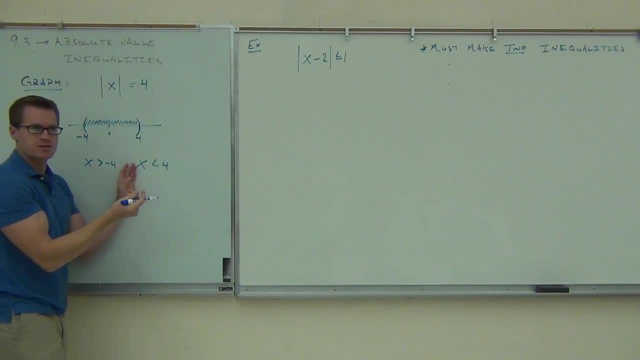 Don't change your problem. just watch up here. If that was an equal sign- we already have done this in this class- you'd have 1 of them equal to 4, and you'd have 1 of them equal to negative 4.. 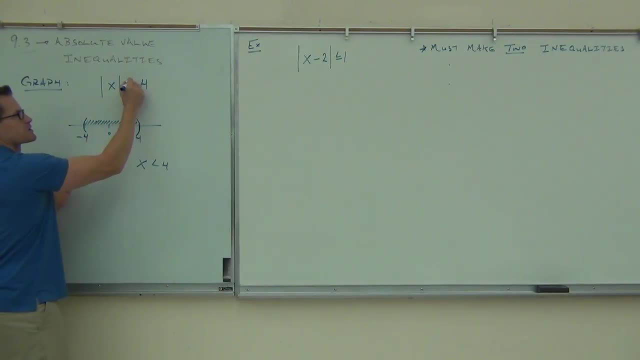 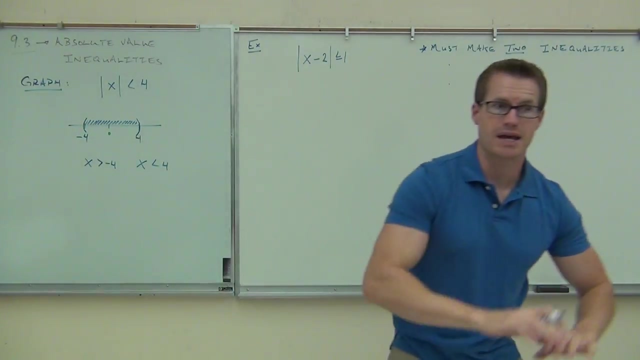 Are you with me? Well now, it's not an equation. It was less than We have, 1 of them, less than 4.. So we're going to make up 1 inequality by not changing any signs at all, just like you did with your equations. 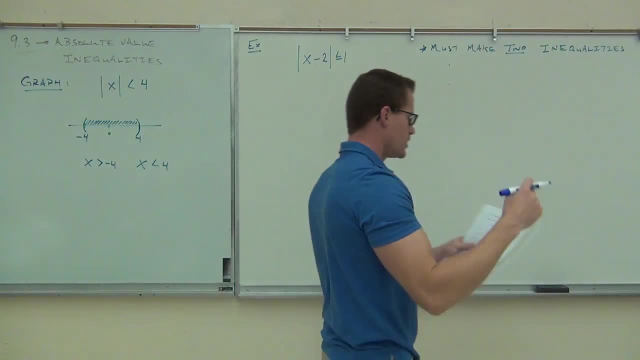 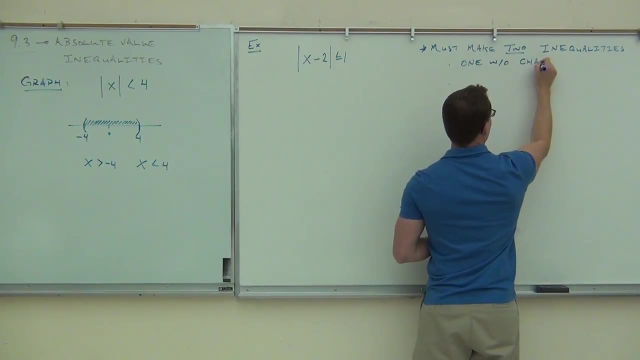 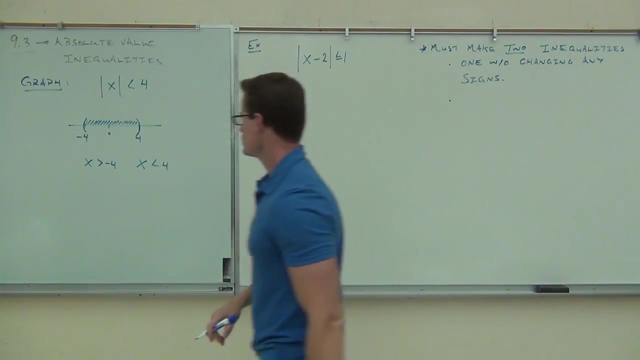 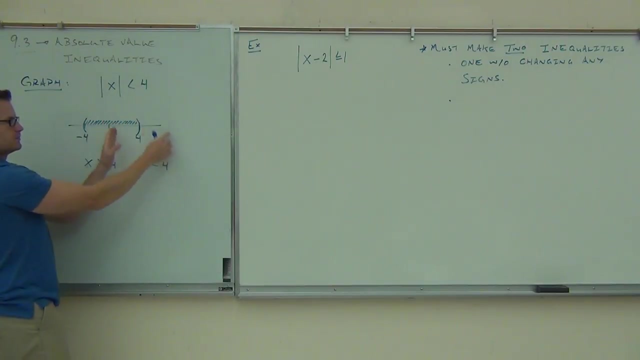 Are you seeing the similarities here? So make up 1 by not changing any signs. Now the second one is kind of important though. Look at the second one. Please watch the difference up here When you made this first inequality. 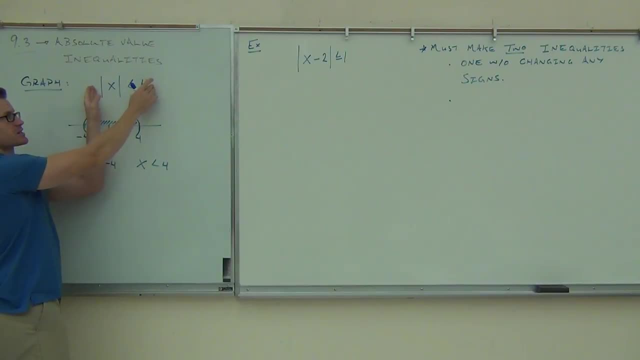 it was very much like making the first equation, where you changed nothing. We said: absolute value of x is less than 4.. Therefore, our first inequality is: x is less than 4.. Now, if this were an equation, I'll go back to the equation. 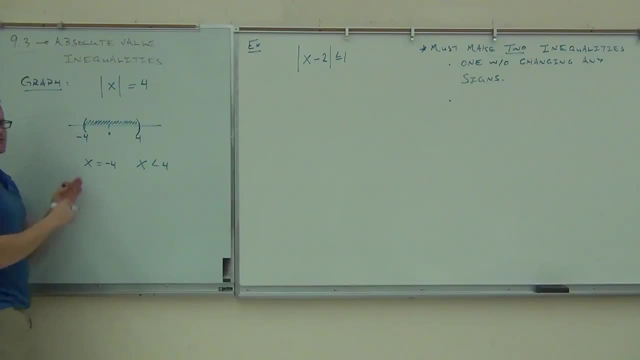 you'd have another x equal negative 4, if that were an equation, right. But look what we're doing, Since this is now an inequality. it's actually not x is. don't write this down, just watch, It's not. x is less than negative 4, is it? 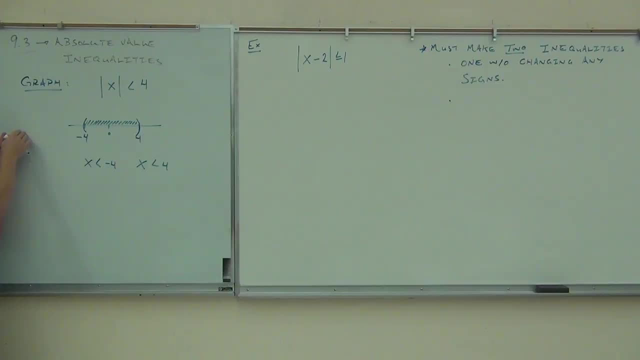 x is less than negative 4, that would be these numbers. We know those didn't work Because when we change them in absolute value, those all become positive and shift them over to that side. They're too big, That doesn't work. 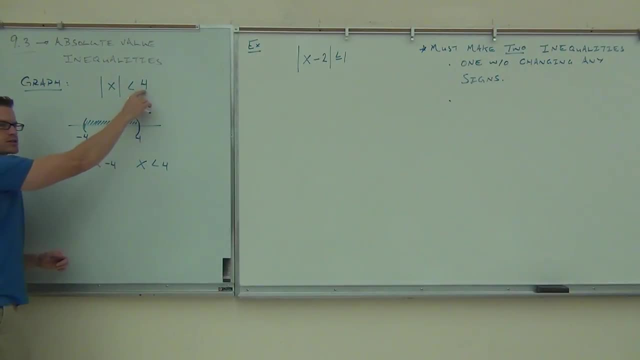 So what happened was, when we changed this number to a negative, we also had to change this sign to the opposite of what it was. Does that make sense to you, Hey, do you remember when you're solving your inequality? what do you do when you multiply or divide by a negative? 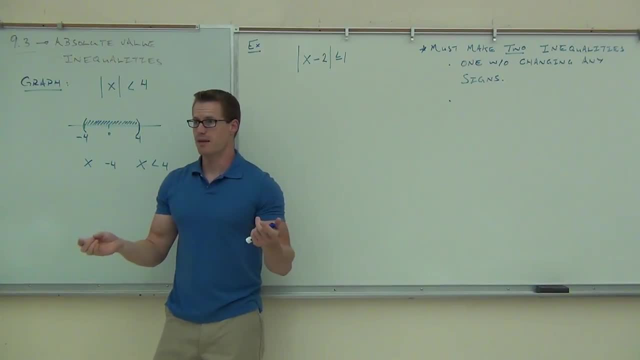 Y'all got to be with me on that. that's old school stuff. Are you with me that whenever you multiply or divide by a negative, you have to flip that inequality True? Look what we're doing. We're essentially changing this sign. 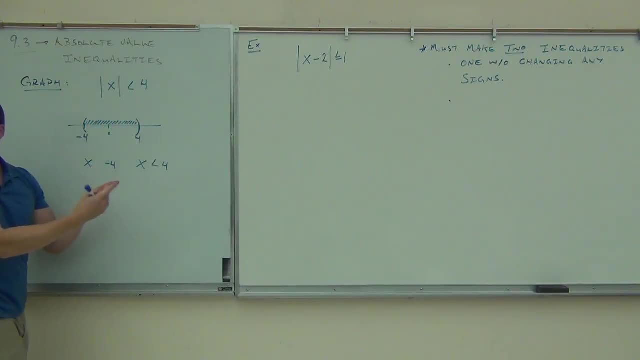 If we are going to change a sign, it's very much like multiplying or dividing by a negative. Here did we change a sign? No, leave it the same. Here, are we changing the sign? Yes, Absolutely. What's got to happen to that inequality? 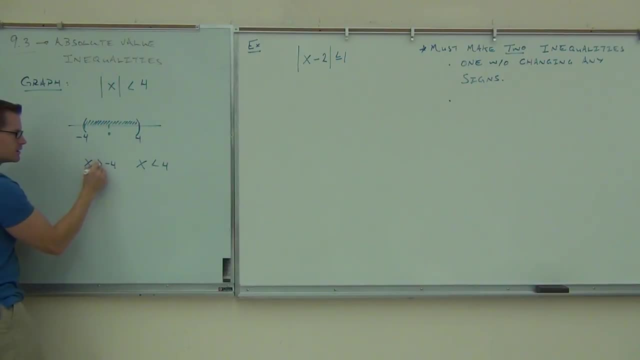 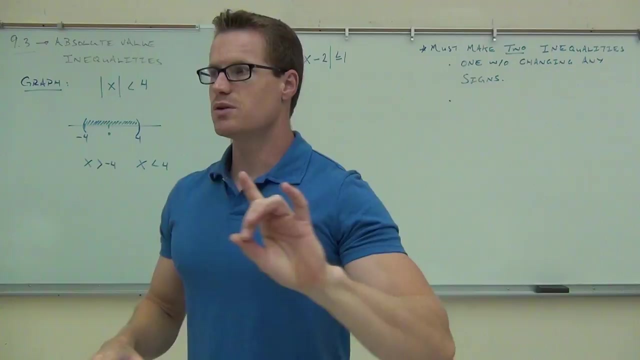 It's got to flip. It's got to flip. Okay, that's where we're getting that thing from. So long story made short. we make two inequalities, just like we did before The first one. we do that without changing any signs. 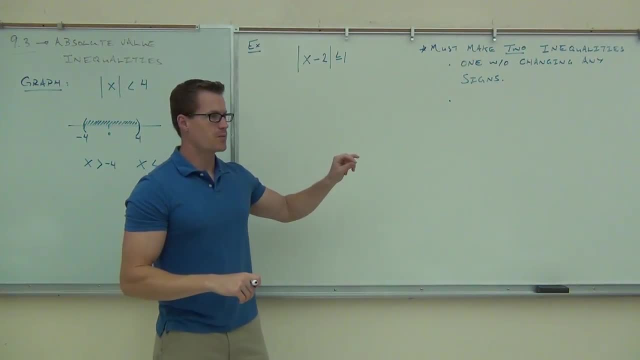 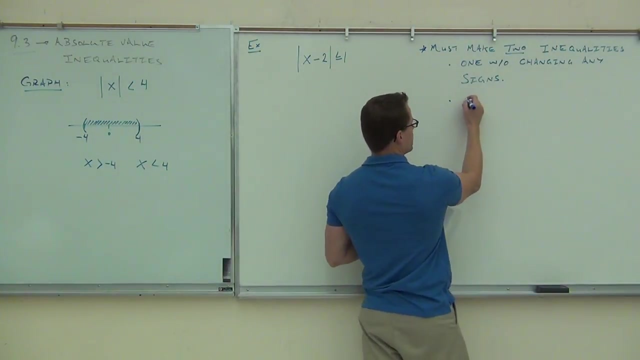 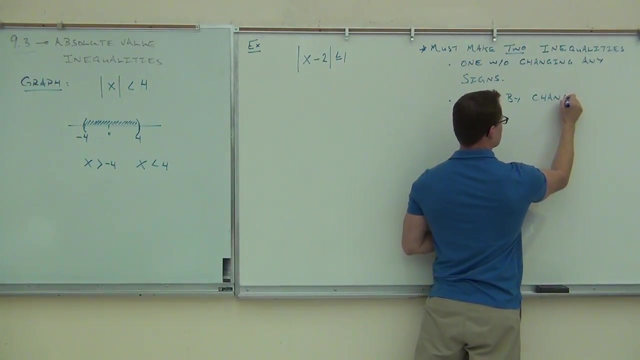 The second one, we change the sign of the number and we flip the inequality. The reason why we flip the inequality is because we're changing the sign of the number. Imagine if you're okay on that. Okay, So one without changing any signs, one by changing the sign, and here's the key point. 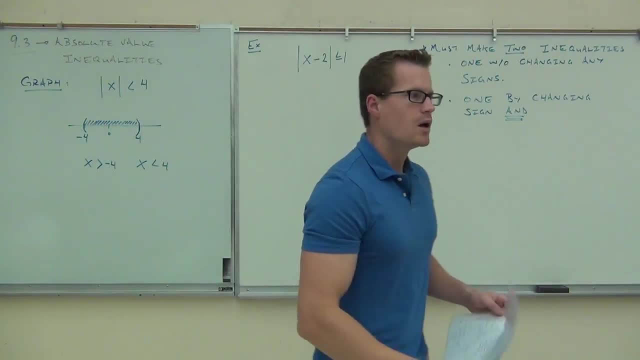 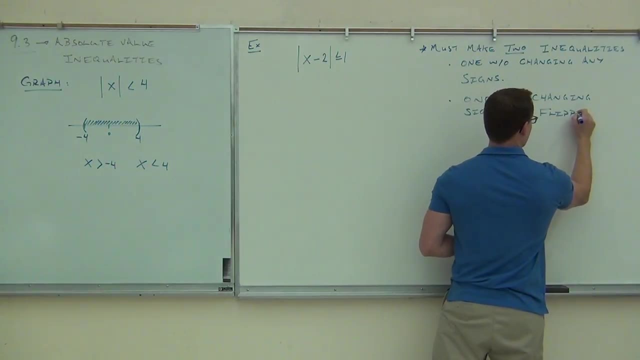 key part of this, because we had that with equations, where you just change a sign, you must flip the inequality. Okay, Hee and停, You want to know what's the UFCb? See what's the US. That's an important part. 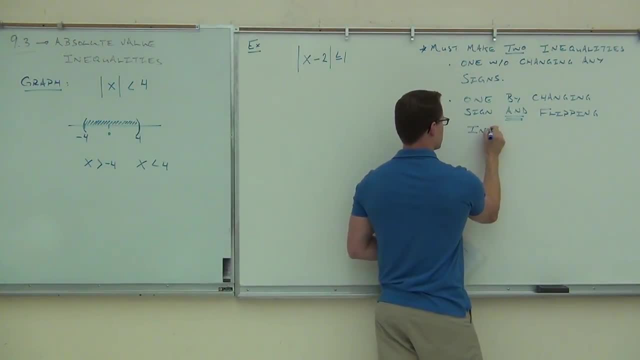 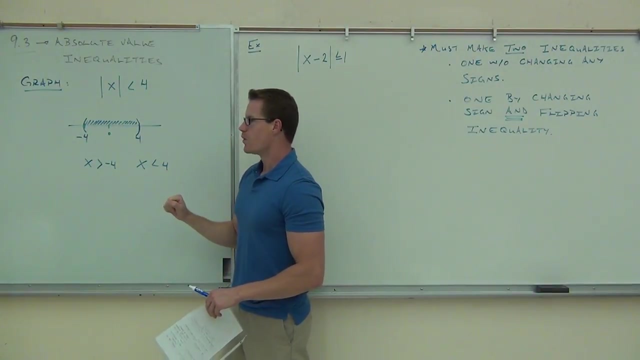 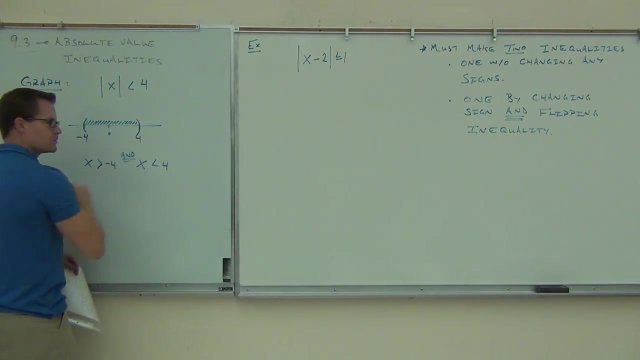 Okay, raise your hands if you're okay with this. so far, and you understood this, this example over here, That's good. Okay, so we know, these are the numbers between negative 4 and 4, or in other words, the numbers less than 4- and we saw that word and that's where that's coming from- and greater than. 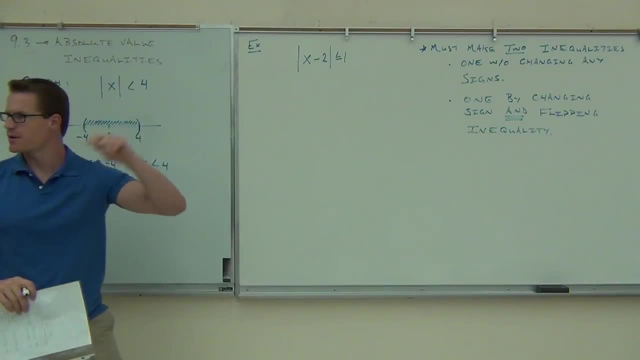 negative 4.. It's between there. That's where the and is that crossover? Notice how we have a crossover here. Now I want to show you one thing. I'll show it. I'll make up the two equations I. 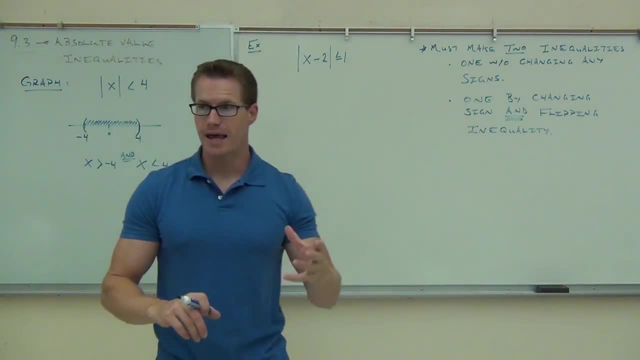 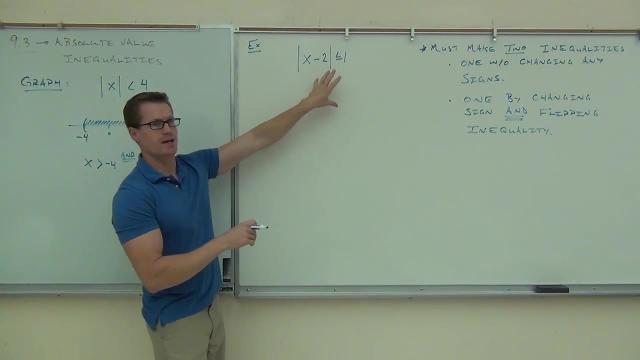 want to show you something on both of these things: what we can do with our and or our absolute value inequalities. Check this out. Firstly, how many inequalities are we going to make out of this thing? Good, The first one is one where I'm not going to change anything about it. 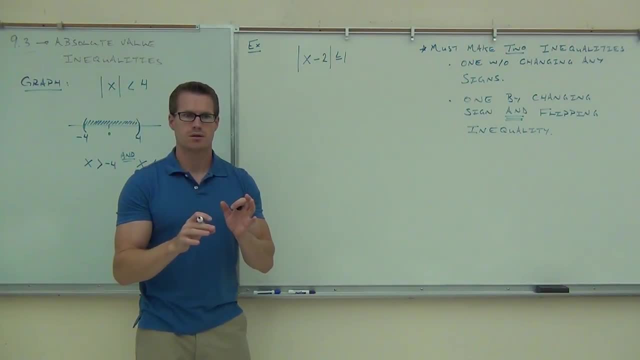 so can you tell me exactly what I'm going to have for my first one, X minus 2, and what Less than or equal to 1.. Perfect First one. I don't change anything. It's just like I get rid of my absolute value. By the way, draw this one on the right side of your paper. 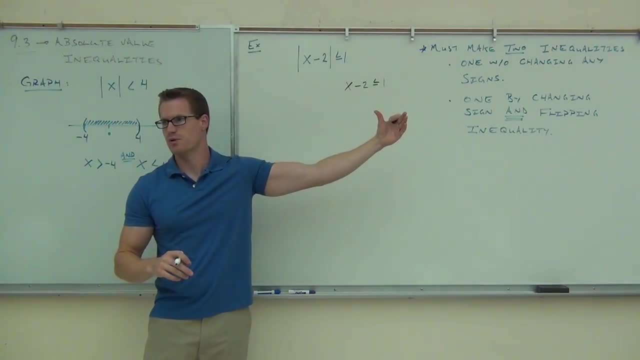 Okay, do the first one on the right side. Trust me on this. It's going to be a lot easier for you to do that. Put this on the right side of your paper. You with me. You'll see why in a little bit. 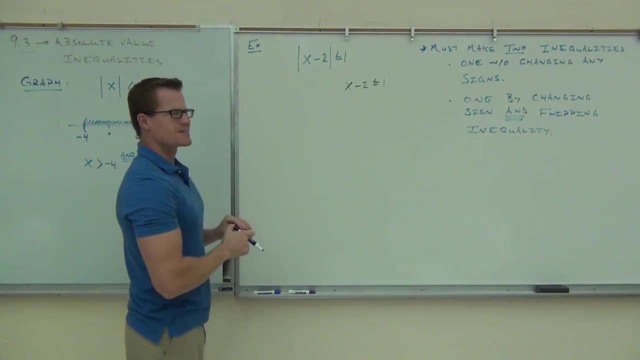 Second one. Second one is going to be: what now? Do I change X minus 2?? Do I change the 1?? What's the 1 become? Tell me the symbol I have to put in between there now. Is it less than or equal? 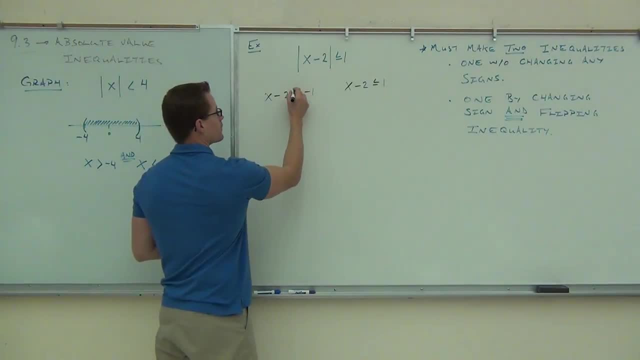 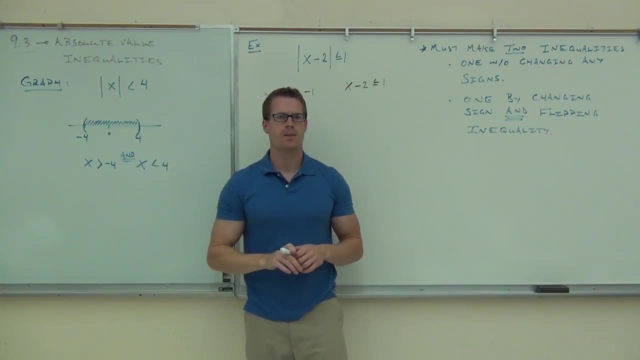 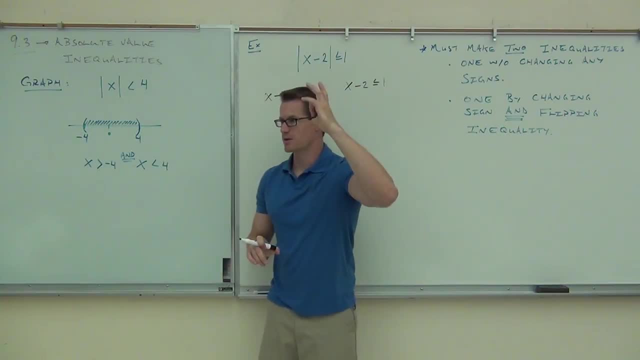 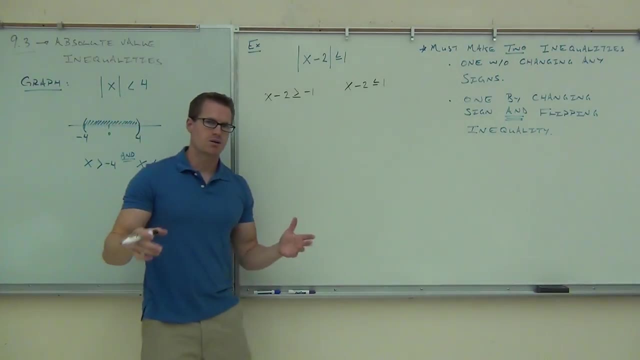 Okay. so because I've changed this number to a negative, that means my inequality must flip around. Now there's one cool thing that we can do. I want you to watch over here. Do you remember what I told you about? and inequalities, By the way, this does mean, and just like it meant, and 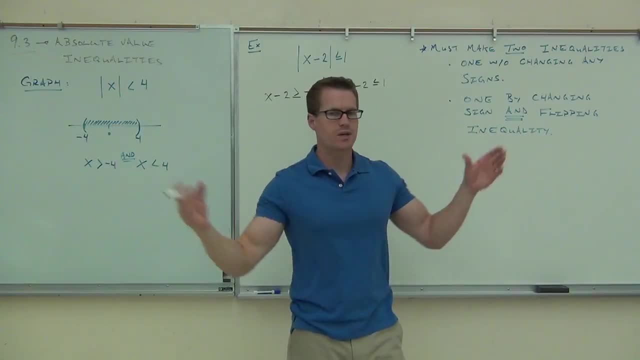 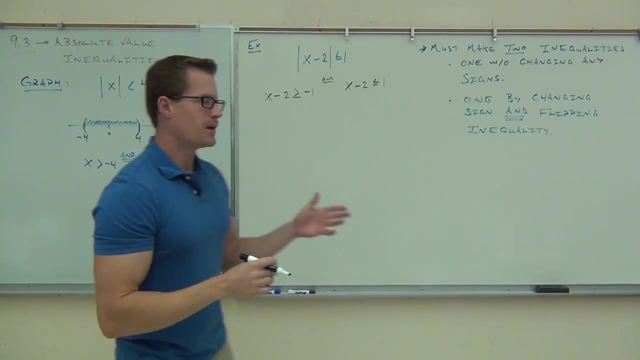 over here. What I told you about and inequalities is that oftentimes we can match them together and make one large inequality out of this thing. Remember me telling you that. Check this out. I'm going to leave this one alone. This is why, by the way, you write this on the right-hand side of your 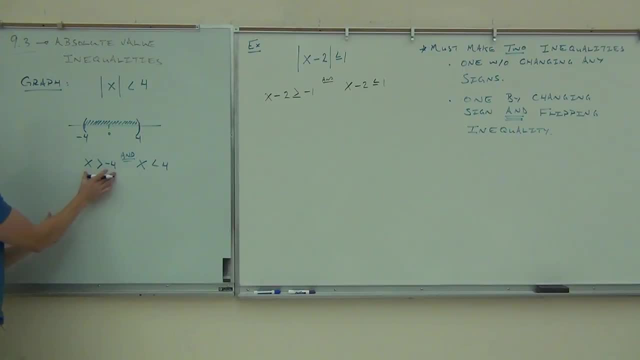 page. I'm going to leave this one alone, but is it okay if I take this off the board and flip it around and put it back? Is that okay with you? So, instead of x is greater than negative 4,, I'm going to have x. I'm sorry, I'm actually. 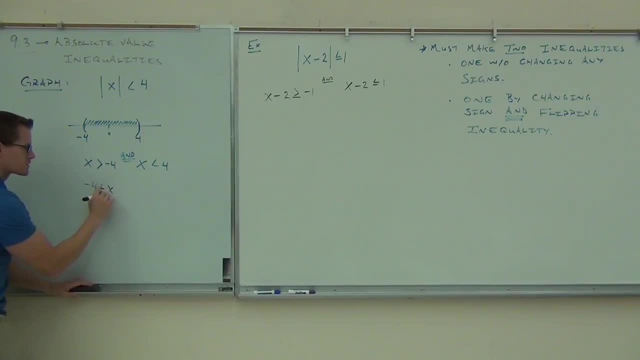 going to flip it around. Negative 4 less than x Do those say the same thing to you, So I just flip this one around. This is the same as that, And x is less than 4.. Hey, is this one of those cases where I can put them together: Negative 4 less than x and x is less than 4.. 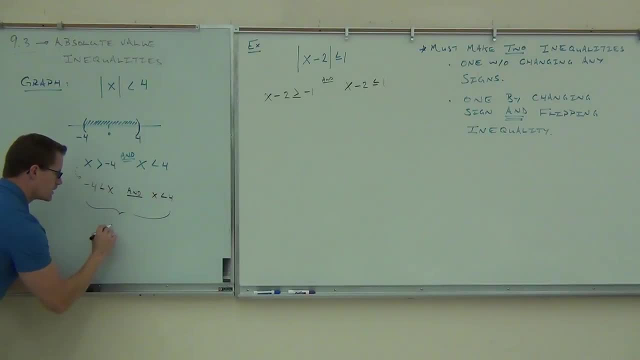 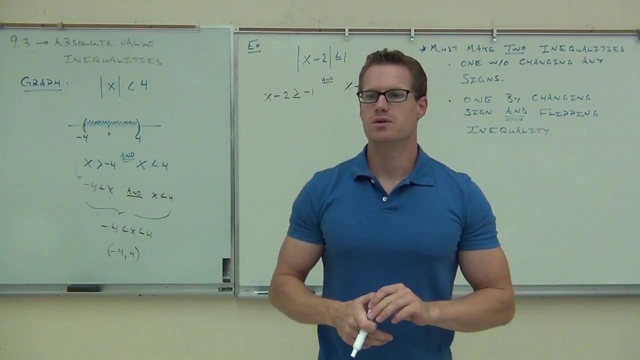 This means negative 4 is less than x is less than 4.. Hey, does this picture look like this picture? It's exactly the same thing. In fact, we can do interval notation. This starts at negative 4, this goes to 4.. We'll use parentheses because that is not equal to, But watch what we can do over. 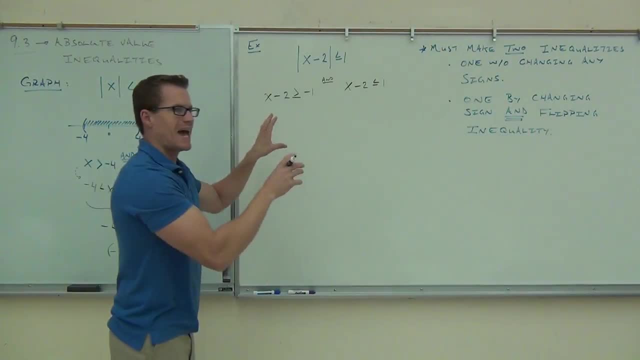 here. This is kind of nice. We can do exactly the same thing here. I want you to follow along with me. Let's take this off the board. Let's flip it around, So, instead of x minus 2 is greater than or equal to negative 1, I'm going to have negative 1. is what now? 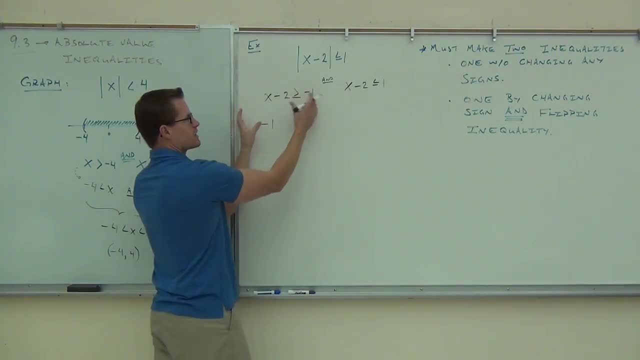 Is it going to be if I'm taking this and flipping it? is it the same? Yes, Is it this way? still No, That wouldn't make sense. This way. Yes, x minus 2.. And x minus 2 is less than or equal to 1.. 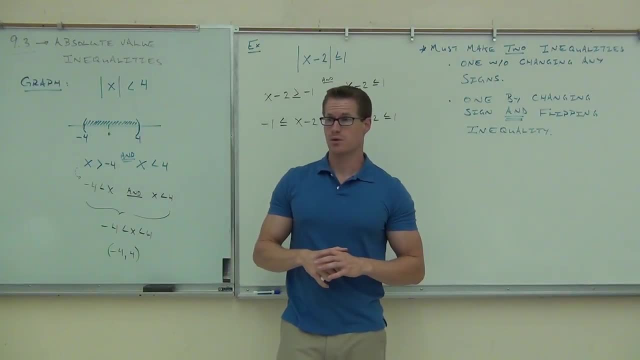 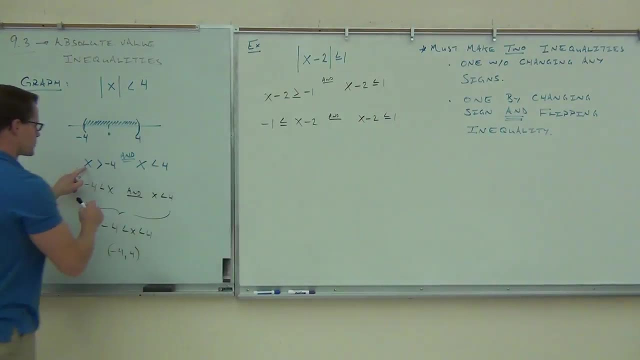 OK, I need a head nod if you guys are OK on doing that Or no. if you're not, You don't change the x minus 2? We don't have to. That's this part of it, The x minus 2, you don't have to do negative 2 plus x. 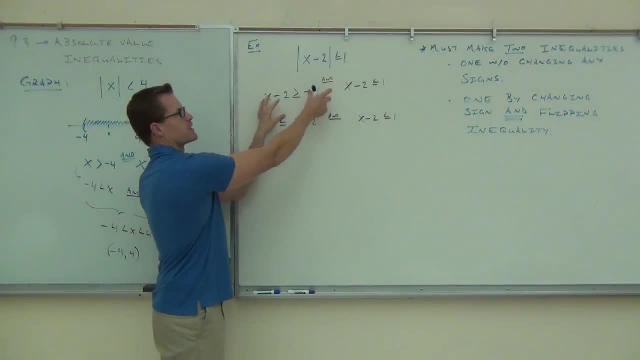 It really doesn't matter. What we're doing is we're just reversing sides here. That's all we're doing. OK, Does that make more sense to you guys? So I've just reversed this. I'm just reversing this one now. 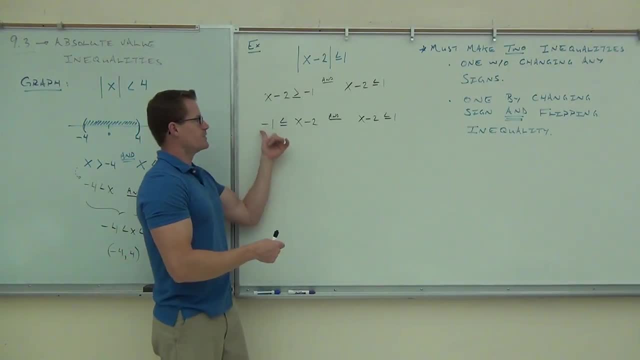 Yes, no, I get a no. Yes, yes, OK, so now we have negative: 1 is less than or equal to x minus 2.. And we also have x minus 2 is less than or equal to 1.. This is the same situation. look at the board as right here. 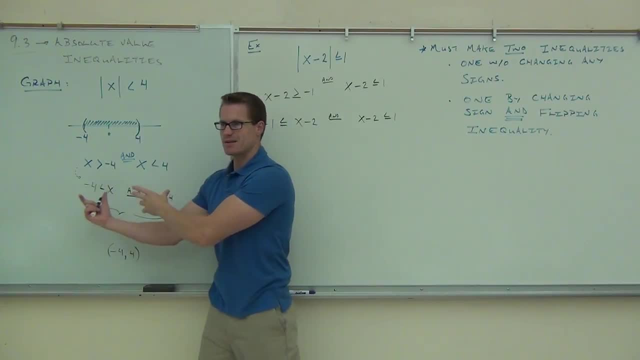 Negative 4 is less than x. x is less than 4.. It's just that instead of x, I have x minus 2.. I can still mash those things together. Check this out, I can do. negative 1 is less than or equal to x minus 2. 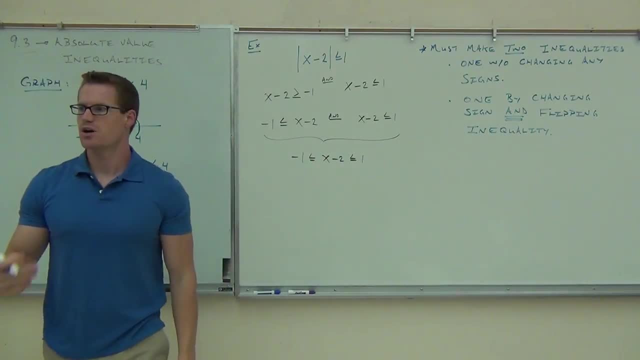 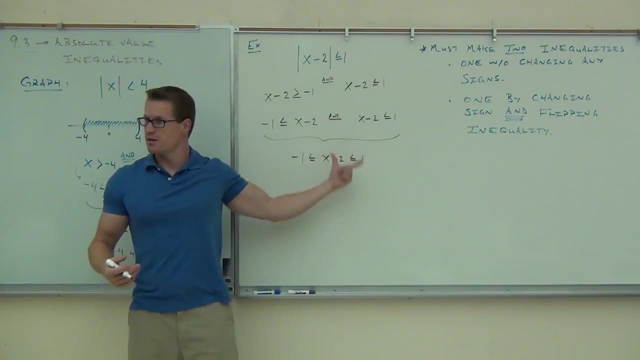 is less than or equal to 1.. I can put those things together and make a large compound inequality out of that. Have we seen stuff like this before? This is why we did it, because I knew we were going to get this situation with our absolute 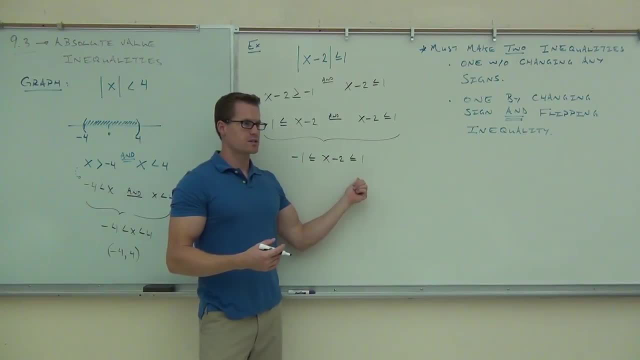 value inequalities. Hey, can you solve this in one step? Yeah, instead of dealing with two different inequalities, with your and, or your less than or equal to or your less than absolute value inequalities, you can set this up like this and do it in one step. 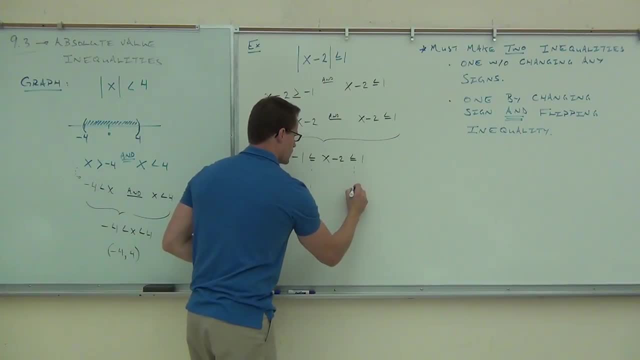 We have our three sections. How are you going to solve this? Are you going to solve this? ladies and gentlemen? If we do that to all three sides, we will have 1 less than or equal to x less than or equal to 3.. 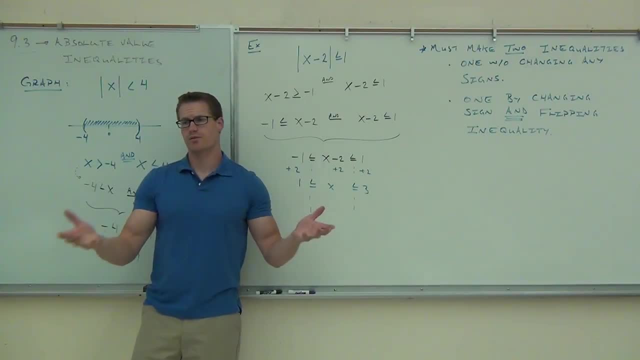 What's awesome about this is you can go directly to your interval notation. Where's this interval? start folks. Where's interval n 3.. My goodness, Brackets, or parentheses here, Brackets. Yeah, you got to be good on that. 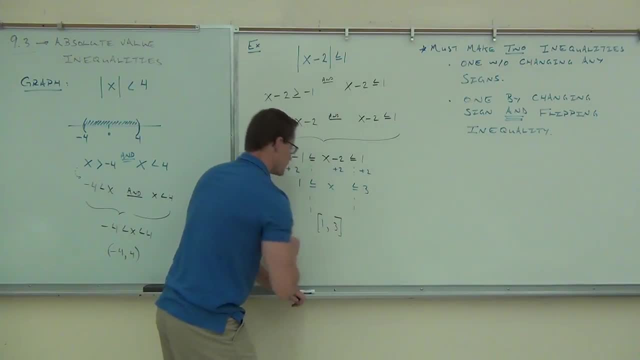 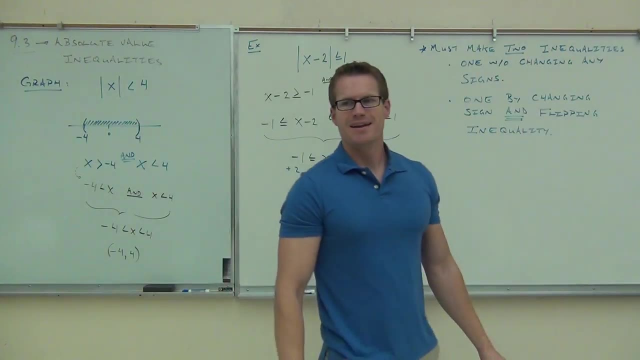 Make sure you're using brackets when you use brackets. OK, Now this is kind of annoying to have to go through this whole thing every single time, right? I don't want to do that. I don't want to do that to you. 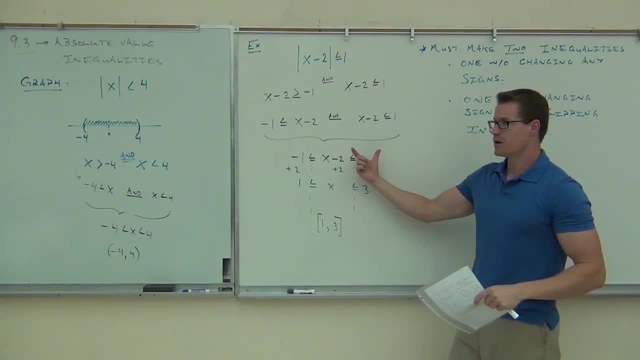 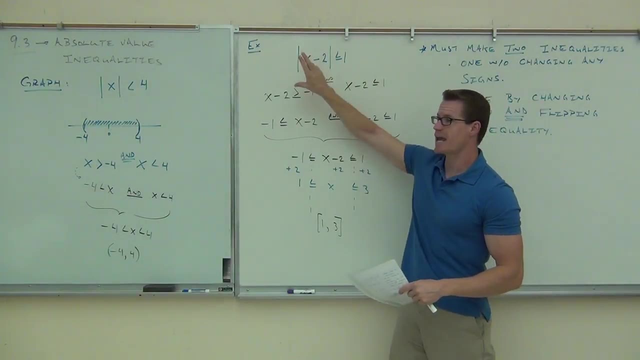 Do you understand how you can go through this every single time? No, I want you to be with it on this. You understand where these two things are coming from, folks. This one: you don't change anything. This one, you change a sign. 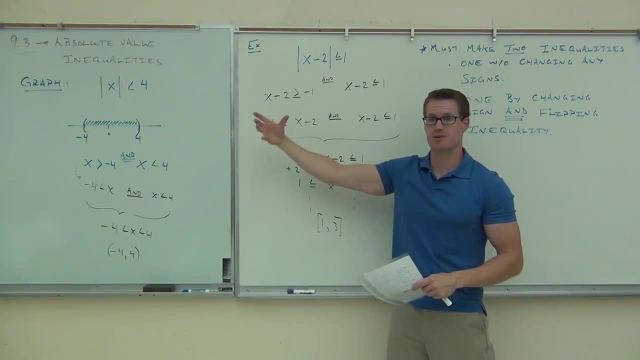 And you flip the inequality. Not your head will be OK with that. That's a must that you have to understand that After this was some manipulation, I picked it off the board and I reversed it, just like I did over there. I noticed that these are exactly the same expression. 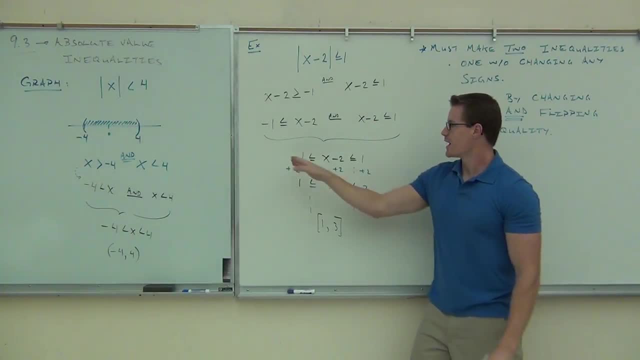 My inequalities are facing the same way. That means I can mash them together and get this expression. Why am I doing that? Well, hey, that's easier to solve right. All I have to do is add 2 to all three sides. 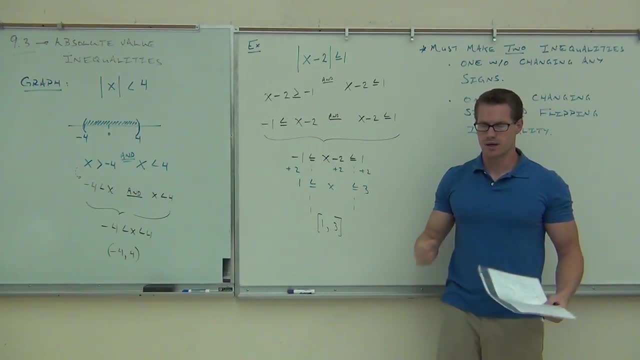 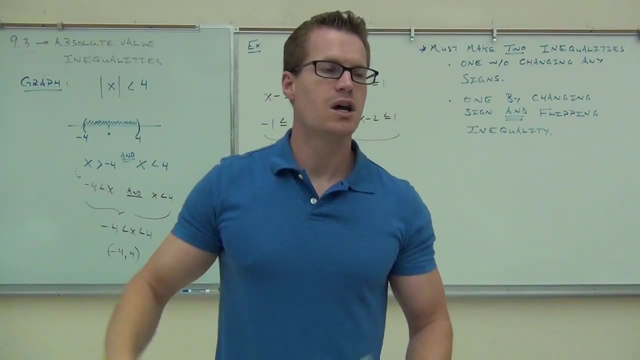 and I'm done with my problem. Yes or no? Yes, OK. Now, instead of doing this every time, we can understand, OK, We can understand that there's a shortcut with these type of inequalities. So here's what I need you to know. 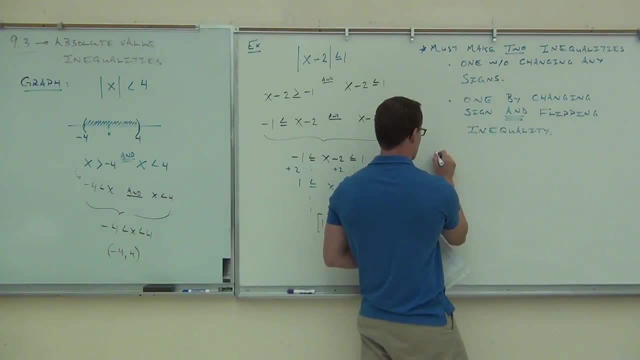 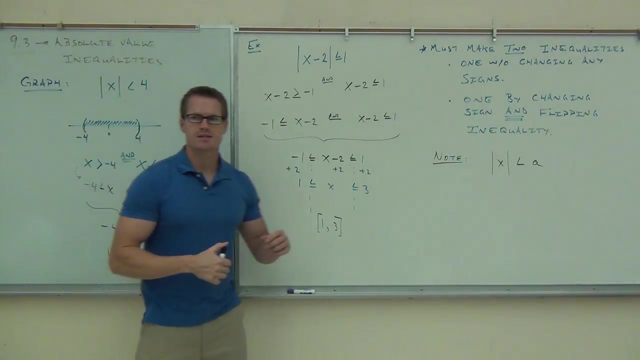 Pay attention: Any time you have an absolute value with a less than or a less than or equal to, any time you have a less than or a less than or equal to something, some number, do you guys see that we'd be able to do this exactly the same way? 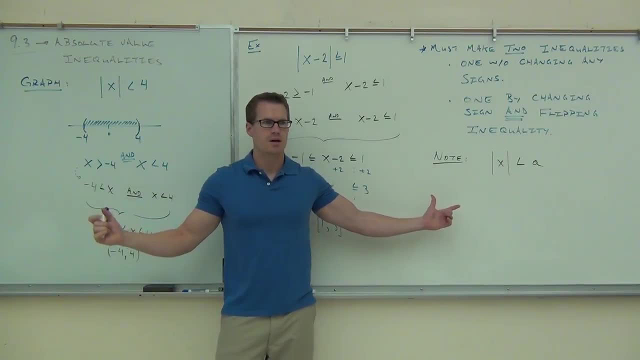 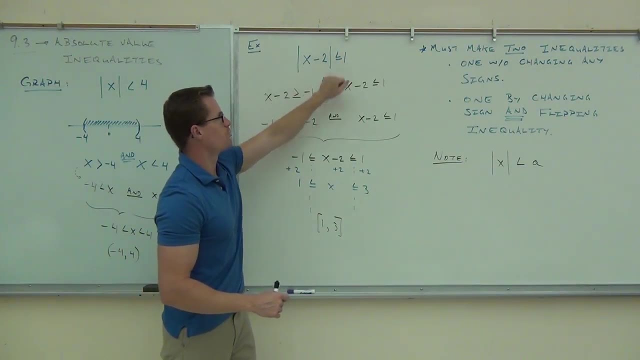 as these examples. Do you see that Every time If we have this symbol, we can write it ultimately as this: We had x minus 2 less than 1.. We were able to, at the very end, write this as negative: 1 less. 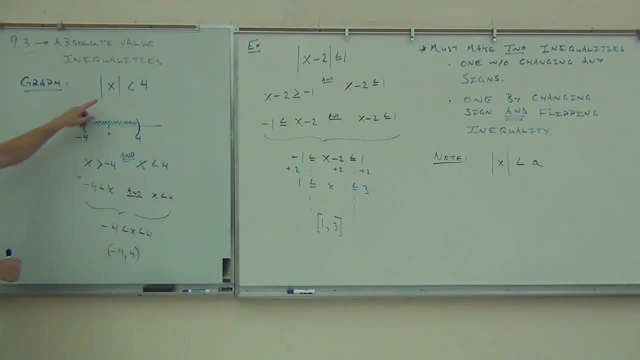 than x minus 2 less than 1.. We could do that. We had it- Absolute value of x less than 4, and we're able to write that as negative: 4 less than x less than 4.. We can do this every single time. 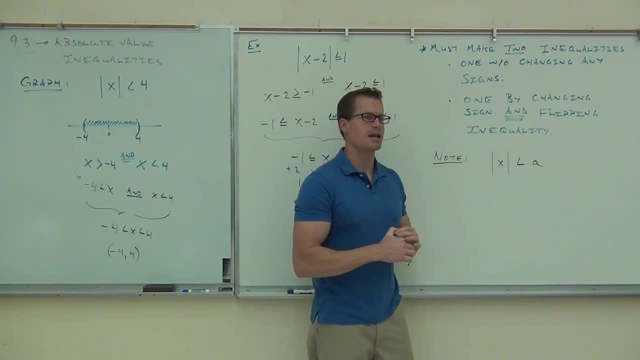 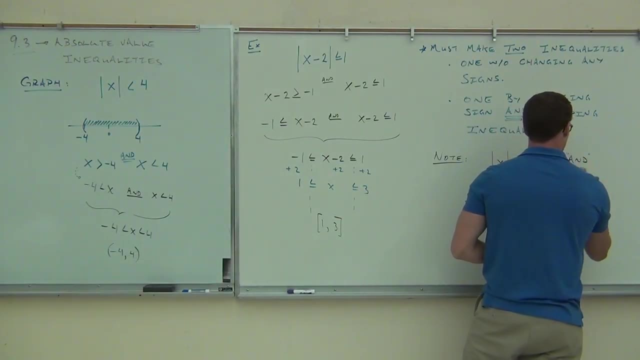 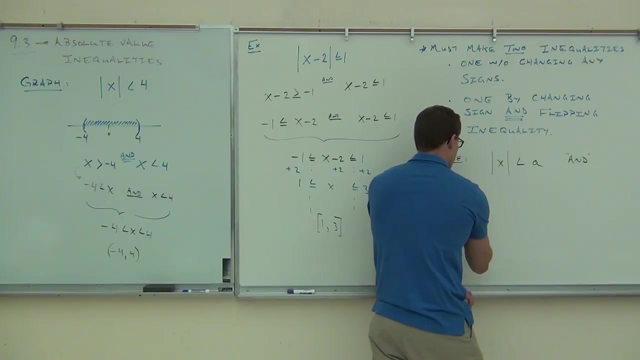 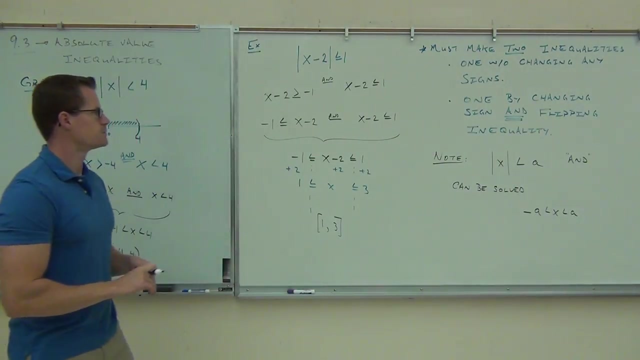 So when you see a less than, it's going to signify an and inequality, Less than is and, Or less than or equal to is and And. we can solve it this way. You know what a lot of people ask. They go, they say, Mr Leonard, but wait a second. 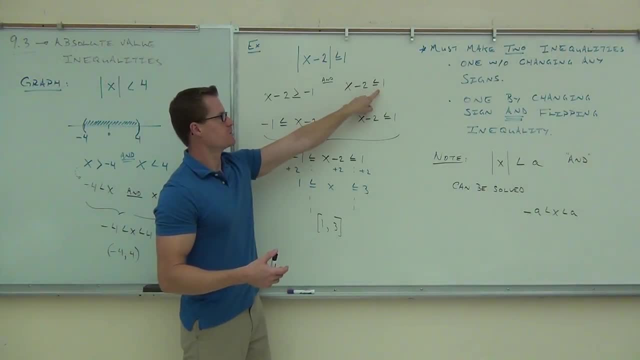 I thought you were going to have two inequalities, And one of them you don't flip the sign. with the other one, you do. And then you- a lot of people ask me: but wait a second, Aren't you not flipping the sign here? 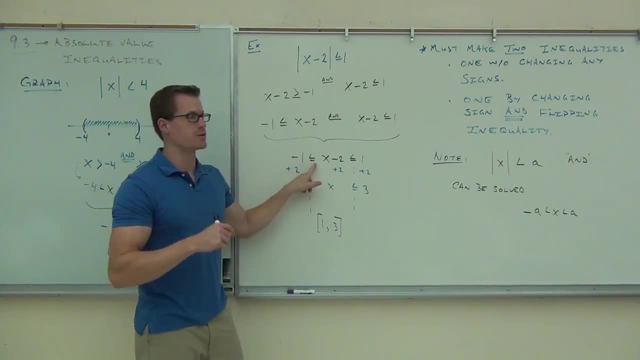 Aren't you not flipping the sign? The answer is yes, you are. I want you to look very carefully at this. You do flip that inequality around- You guys were with me on that right- But then you flip it back around when you change that. 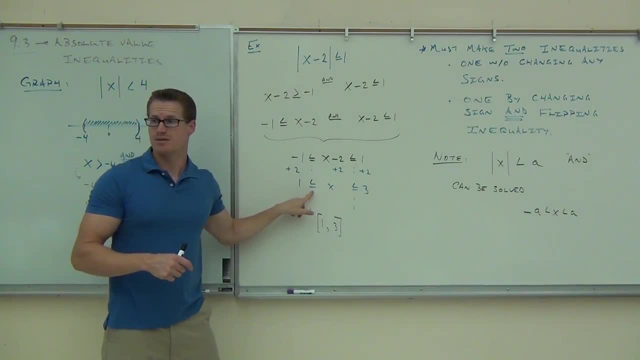 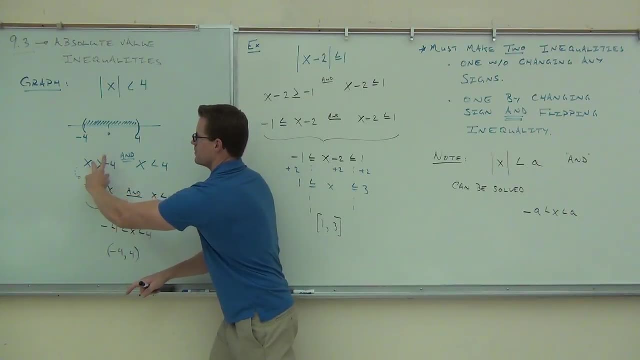 Does that make sense? So is this flipped around? The answer is yeah, it is. It's just you're writing it backwards so it doesn't look that way. Is this one flipped around? Yes, But remember we flipped it back when we wrote it in the reverse order. 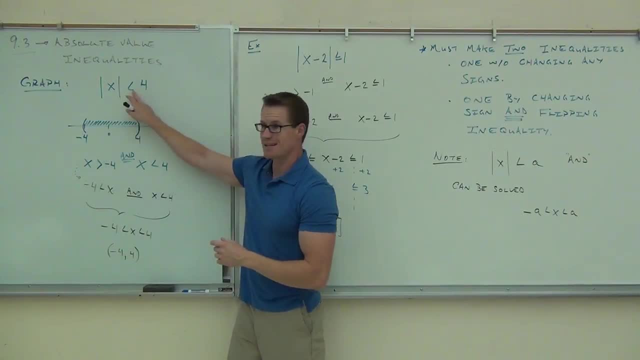 So are these ones written backwards of this? It actually is? It is, but you're flipping it back around. You write it in reverse. That's what makes it look like it's not. Do you want me to flip one side? You flip. you don't flip this one at all. 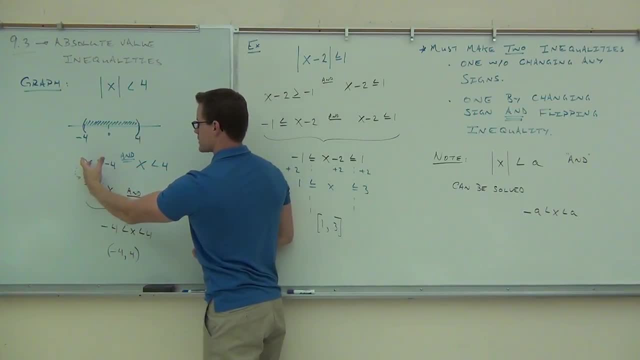 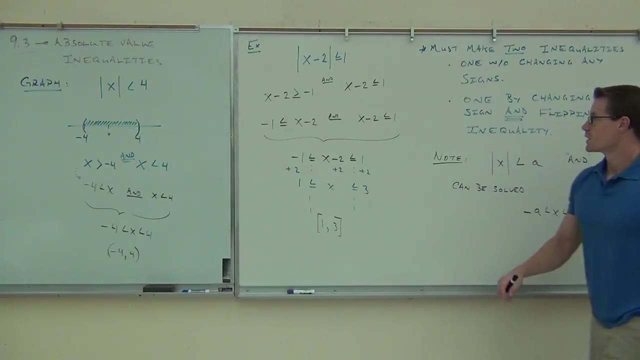 You do flip this one. However, when we're writing this in our shortcut method, we flip it back around So it doesn't look like we're flipping it. So what this all leads to is this idea: We can do a nice shortcut here. 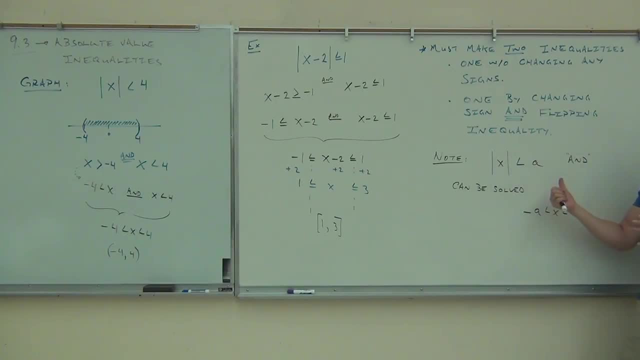 If we have an absolute value that's less than or less than or equal to some number, we can write this as negative. We're changing the sign, We're flipping the inequality, But we're flipping the inequality, But we're flipping it back. 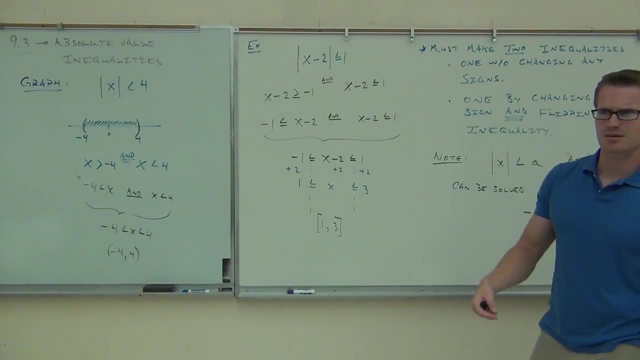 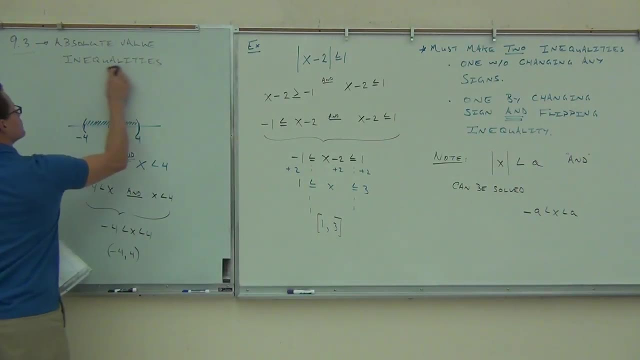 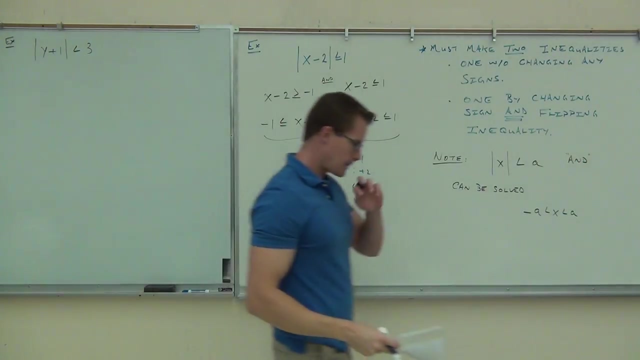 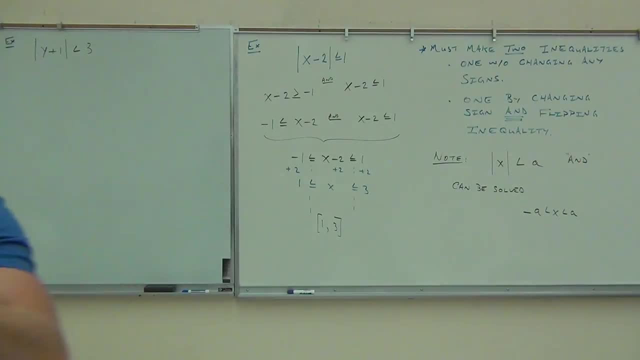 Let's do that. Okay, I need to be rock solid on these two questions. First, does it fit the criteria for doing this for our shortcut? Does it fit the shortcut method? Or in other words, is it an and inequality? Yes, 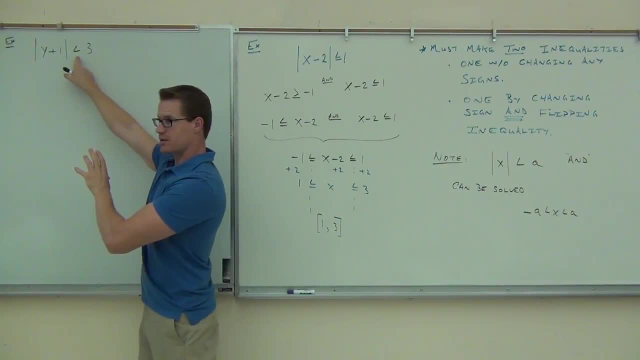 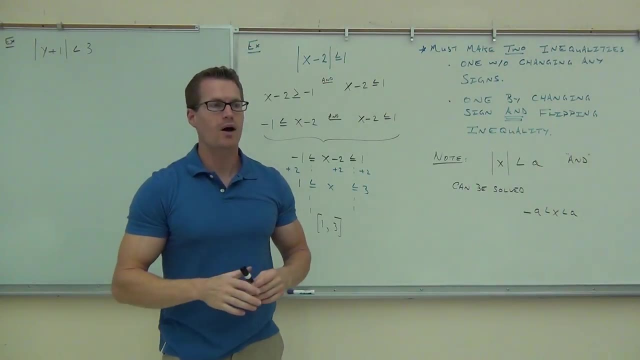 Yes, This means, and This means that you're going to have our less than, or less than. equal to means our, and It fits the criteria because it is our less than. Are you with me on that? This is less than. In a little while, we're going to have greater than. 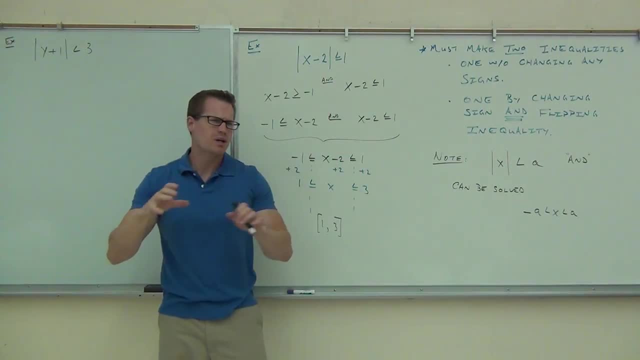 It's not going to fit this. We're not going to be able to do the same thing. So you need to really kind of get that with the less than or lesser equal to, we can do this. If it's not this way, we cannot do this. 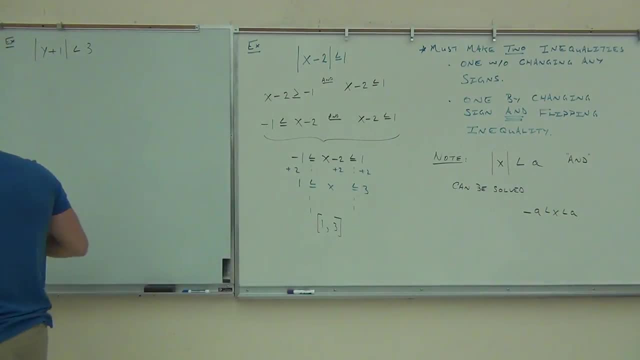 Measure W within that. Okay. So since this fits our criteria, let's do what this shortcut says it can do. What's the first thing we're going to write then? in this case, What now? Negative 3.. So this says that I can write negative A, A and put X in the middle of it. 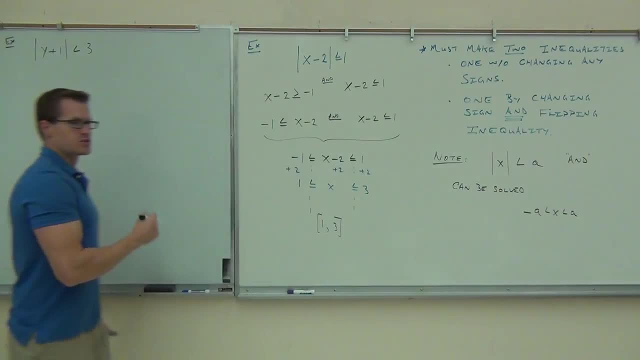 Basically, that's what that says. So I'm going to take my. in this case, A is 3.. So I'm going to put negative 3.. Remember that, folks. what we're really doing is we're writing two inequalities, right? 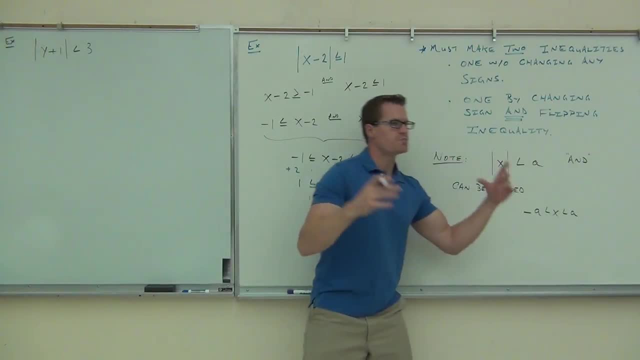 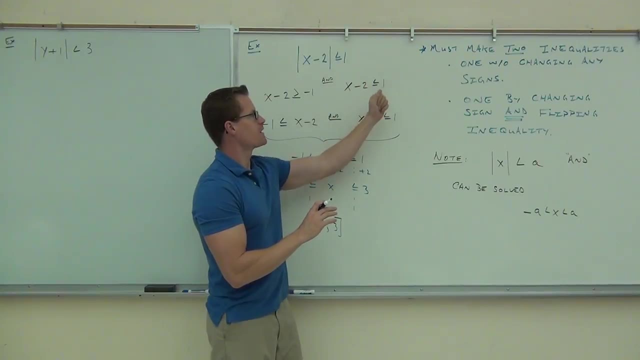 We really are. Look it, Here's one of them, Here's another. We're just mashing them together. So we still have to write two inequalities. We're still doing inequalities the same way. We're writing the positive of that number and the negative of that number. 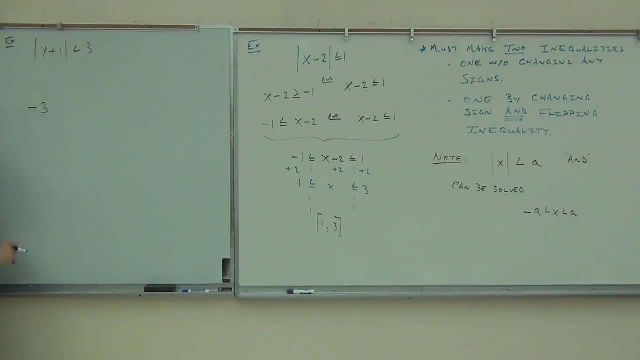 So we are still going to write negative 3, and we're going to write 3.. What goes in the middle of those things? If you're a little confused on this, pay attention up here. okay, Now did you kind of buy into the fact that we need two inequalities? 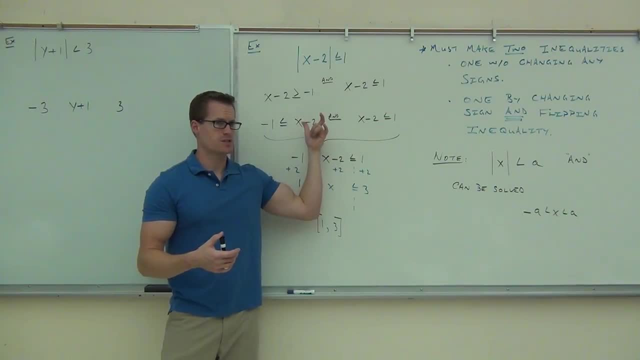 Did you buy into the fact? Did you buy into the fact that one of them's got to be positive, one's got to be negative? Same thing as you did with your equation in your homework. Did you follow me? that one inequality we keep exactly the same. 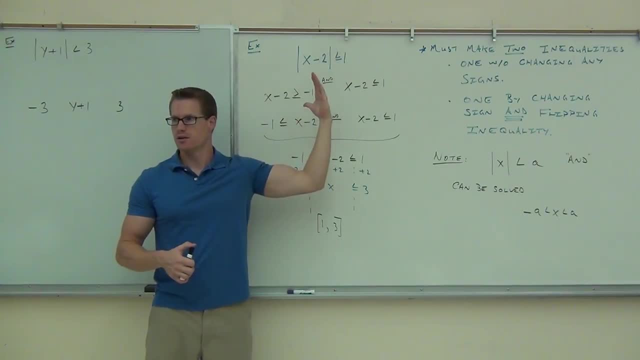 but the other one. we have to flip it around because we're changing the sign. Keep on doing that. Now I want you to watch what happens. We are going to make two inequalities here. Check this out. Ignore this for a second. 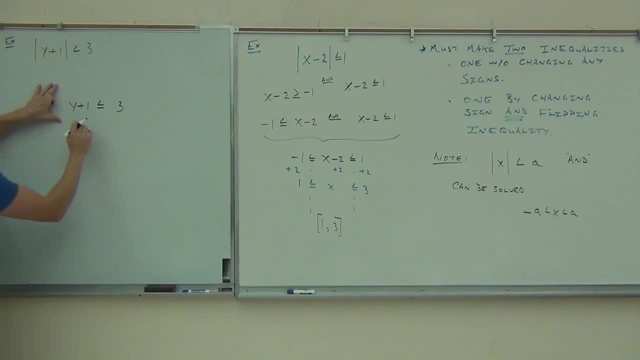 Can you see that this is our first inequality? Oops, That's not our first one. That one is: Can you see that that's our first inequality? Okay, you ready? Now ignore this side for a second. Can you see that I'm going to flip this around and make it? 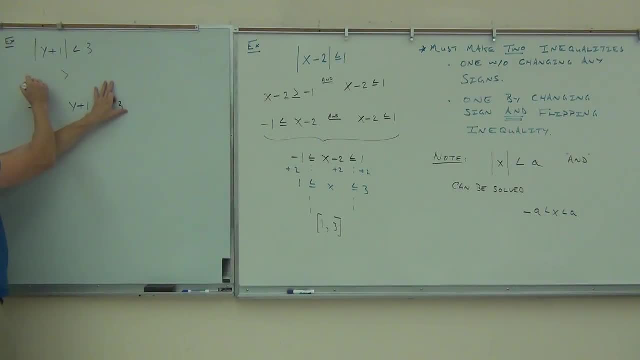 I would have made it going this way right, But it would have been: y plus 1 is greater than negative 3, true. Now, in order to get it to this form, I have to pick it off the board and flip it around, true. 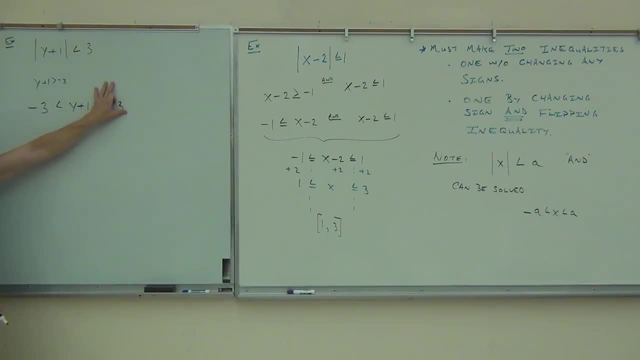 Mm-hmm, That's going to change. That's going to change us back to this way. That's why that's that direction. Does that make sense? So am I making two inequalities when I do this? Yes, here's one, here's two. 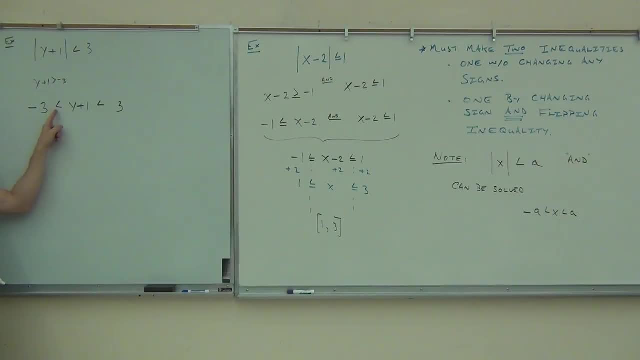 Am I changing the signs of the numbers? Yes, here it is. Am I writing this in the reverse order? Yes, I am, but I'm flipping it back around when I write this in this particular way. Raise your hand if you understand that. 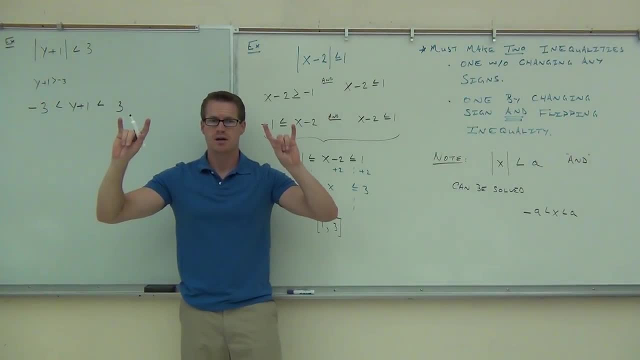 Good, You have to understand all those ideas that I'm writing two inequalities, that one's positive, one's negative, and that I'm flipping the sign when I make that, flipping the inequality when I make that. But why do we do it this way? 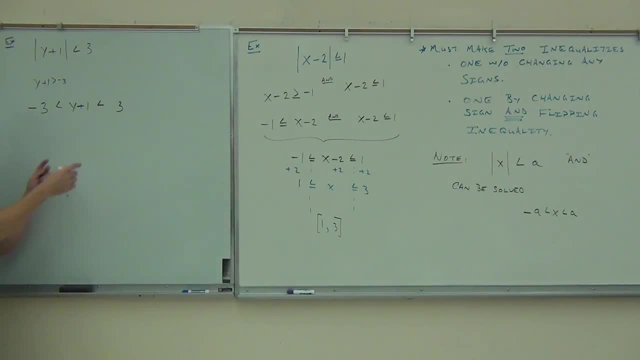 Well, this is a lot easier to solve than doing two inequalities and it's already an interval notation. That's what we like. So when we do this problem, how do I get y by itself first? Okay, let's do that negative 4, I'm not going to change any inequalities- y less than 2.. 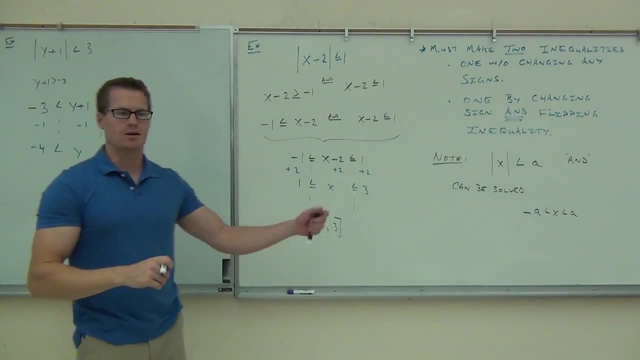 That's beautiful. It's already set up an interval notation for me. I don't have to do anything else. All I have to do is tell where it starts, Tell me, Tell me where it ends. Use the appropriate symbols. We're good. 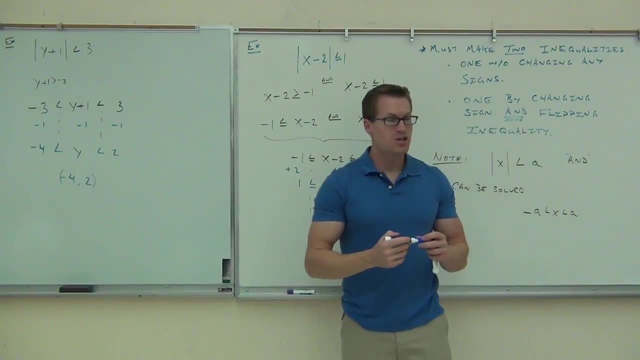 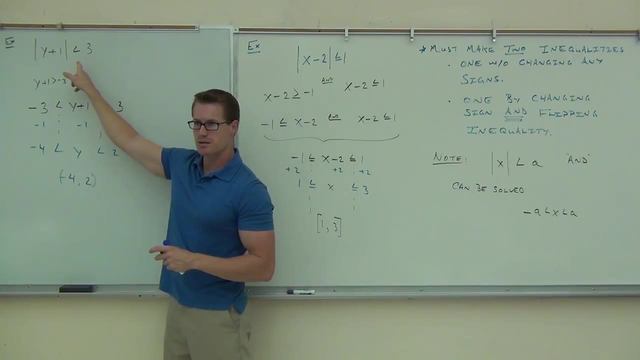 Like it. Not too bad, right, Not too bad. You just have to remember one thing With this: less than or less than or equal to, you can do this. If this is not less than or less than or equal to, you can't do this. 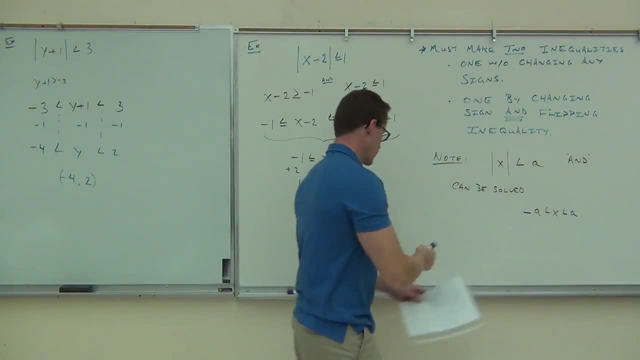 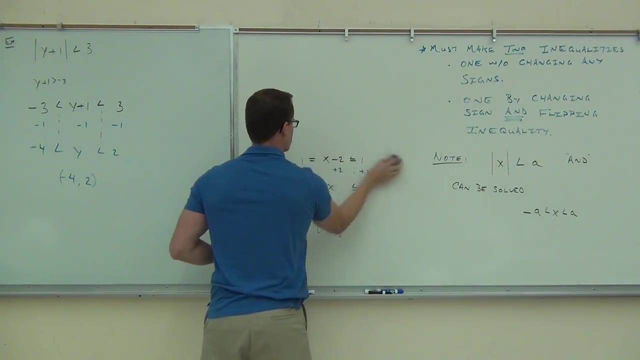 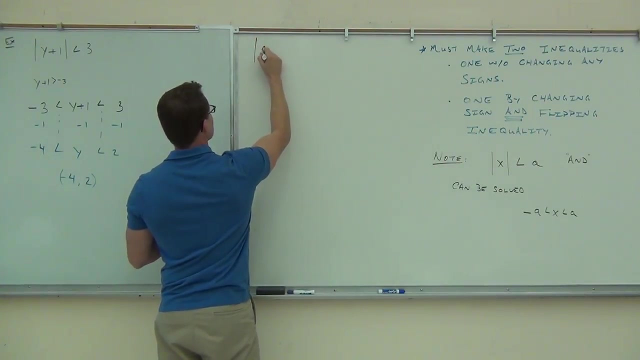 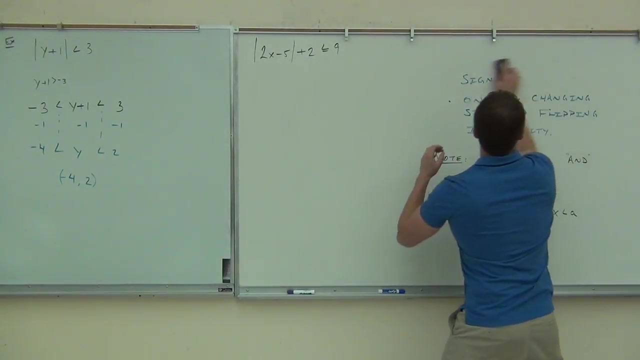 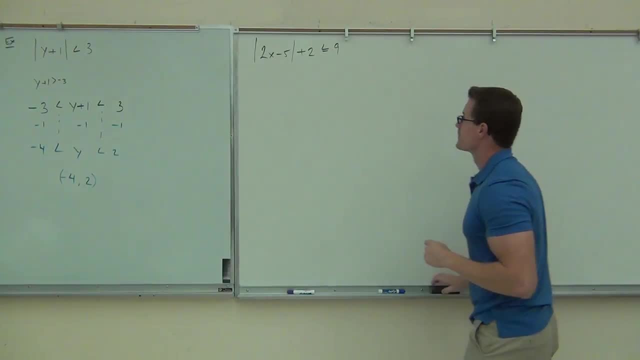 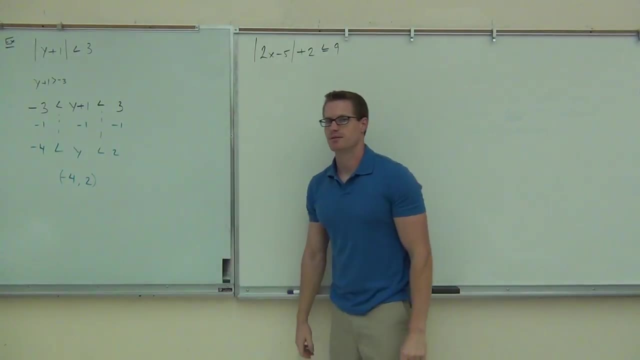 Thank you. Now I have to take a look at how to do this, to take a good long look at that. That should look kind of familiar to you from your homework. What's the first thing you might want to do here? Say it again. 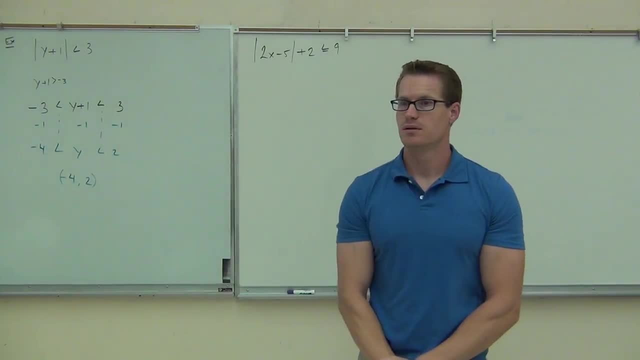 Subtract 2.. Why subtract 2? Because you're Aha, So the same rules apply, Same rules. Remember on your equations, on your homework, how you isolated the absolute value. You got it to the absolute value first, before you made your two equations. 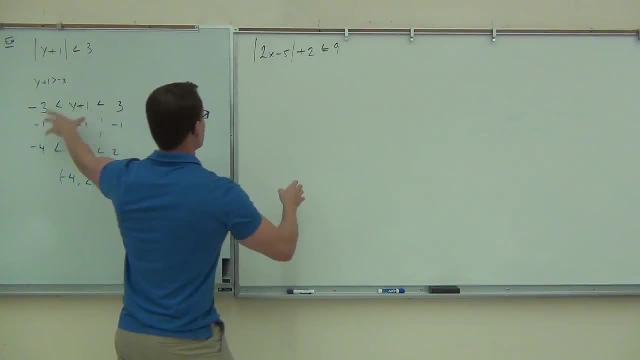 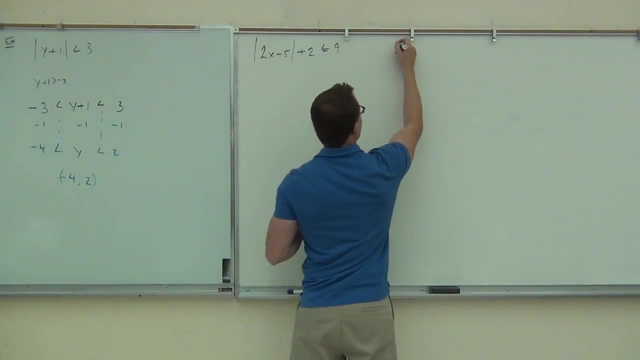 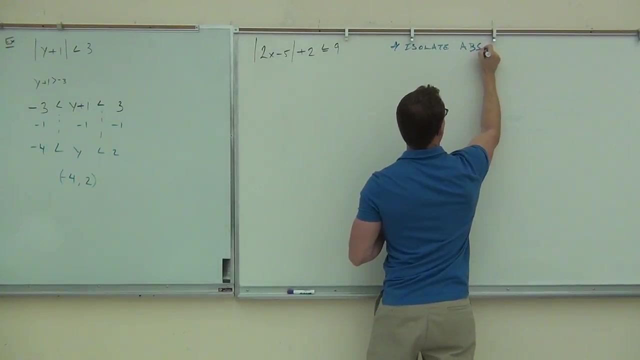 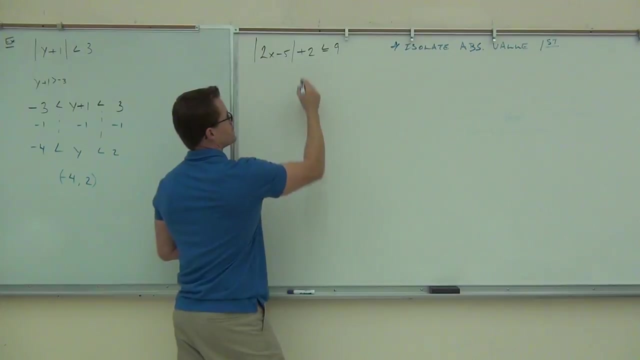 Same thing happens here. You cannot go directly to this part if you do not have an absolute value all by itself. So, just like with your equations: hey, isolate the absolute value, Isolate the absolute value first. So of course, yeah, in this case we're going to subtract 2.. 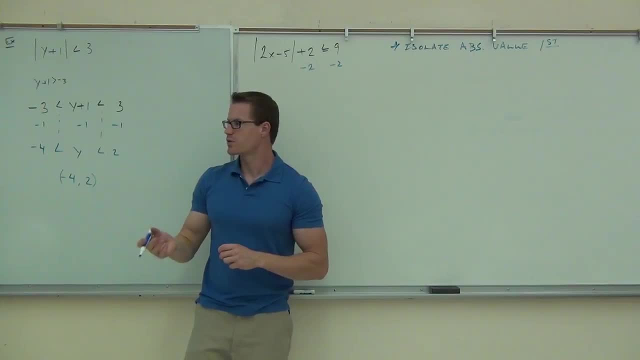 That's a really important point. If you don't do that, one side is going to be off. Your left side of your expression is going to be off. So we'll have absolute value of 2x minus 5 less than or equal to 7.. 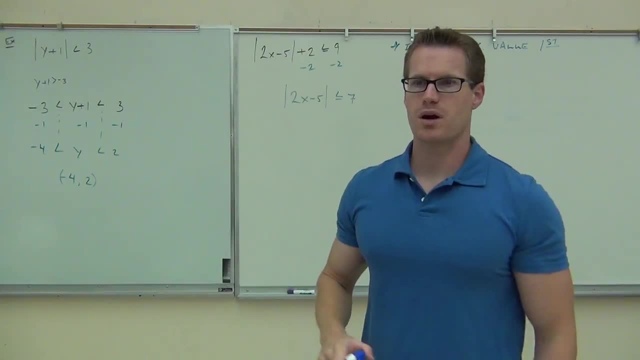 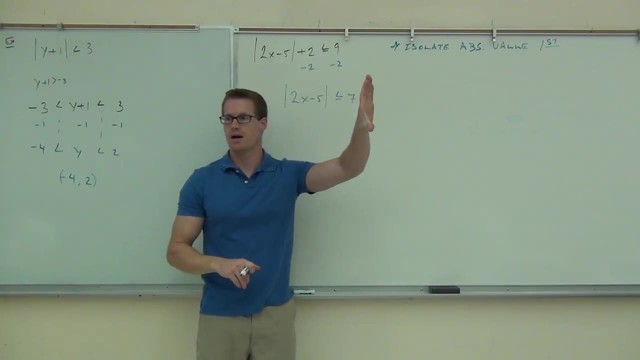 Okay, everybody Up here, Is our shortcut going to work for this problem? Is this an? and inequality? Yes, Look at it. That's a shortcut right there that says it's less than or less than or equal to. That means that, instead of doing my two inequalities separately, 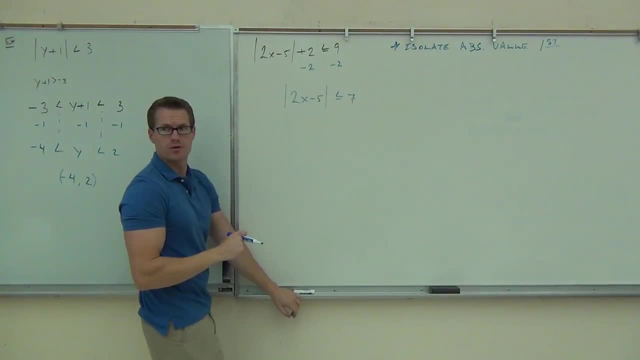 I can make two inequalities together. Tell me how to start this. What number do I write first? What symbol? now And again last time I'm going to explain this, Even though this looks the same, we are writing it backwards, It's just, we're writing it backwards. 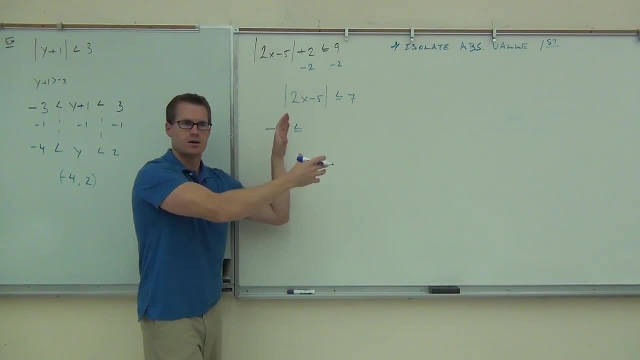 We're writing it in the reverse order so it flips it back around. Not sure if you're okay with that. Okay, And what goes in the middle? 2x minus 5. Is less than or equal to what 7.. 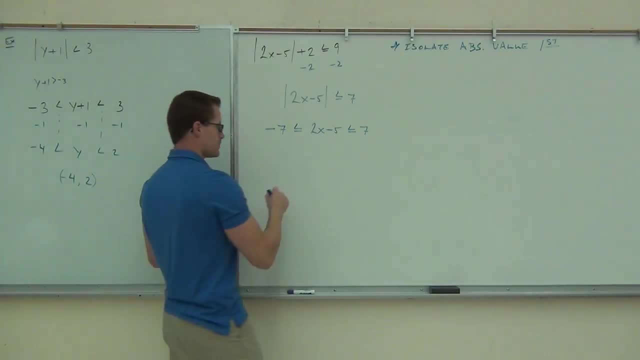 Good That we can solve pretty easily. How do we solve that? Add 5 to the other side, Add 5.. So add 5 pretty much everywhere. I know this is negative: 2, less than or equal to 2x less than or equal to 12.. 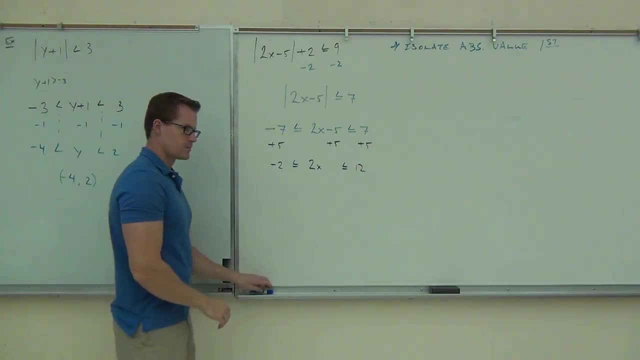 And our last step, ladies and gentlemen, Divide it by 3.. Negative: do I flip the signs around. if I divide by 2? It's not really division, it's division by a negative. that would do that. So, negative: 1,, less than or equal to x, less than or equal to 6.. 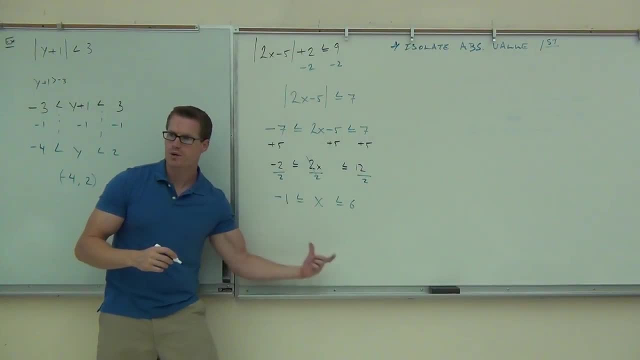 This is great. I want you to use a shortcut, because this is already an interval notation, practically for you. It's already done. You don't even have to draw a number line. Well, you can if you want to, but this is done for you. 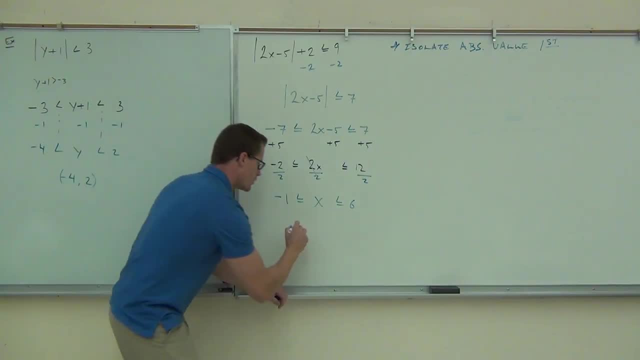 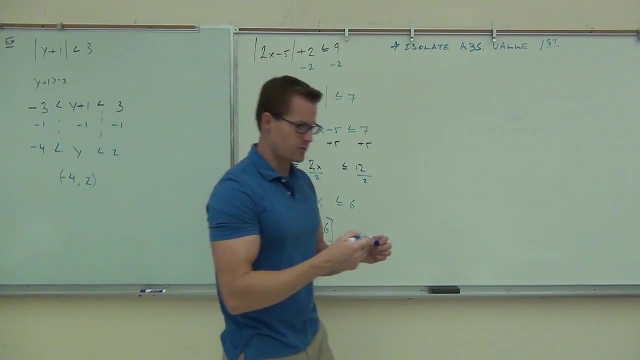 Do you see that right? It's kind of nice. Where does it start? Negative 1. Where's your name? 6th day: Brackets parentheses. Brackets parentheses Because we have those equals. 2, we've already done that, that stuff, several times. 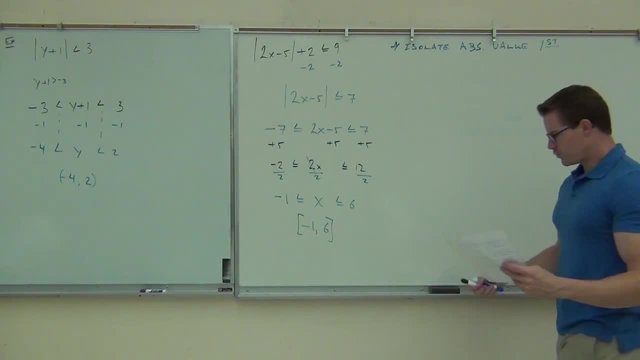 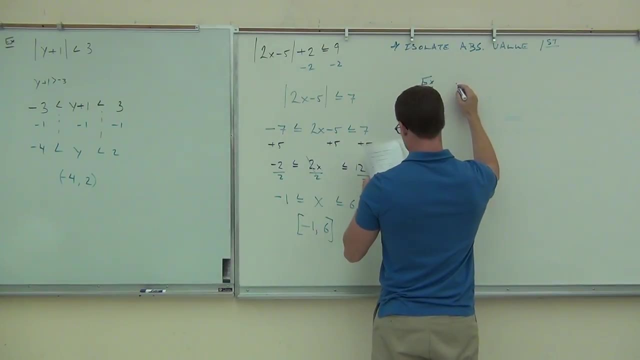 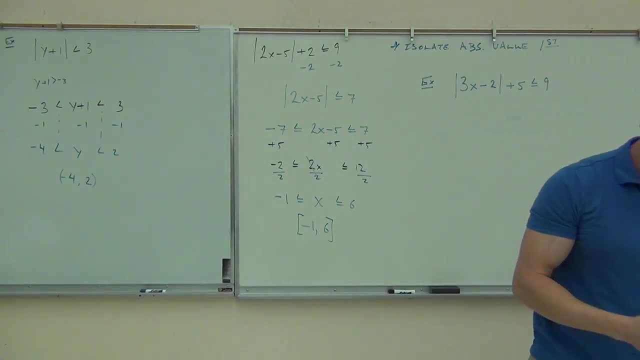 That should be familiar to you. We can do that. Okay, give one of these a try on your own, would you? Yes, Okay, it's going to be all right. Okay, Is this for me? Yes, Okay, All right. 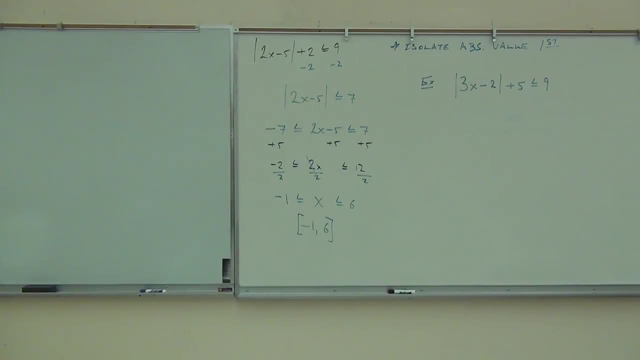 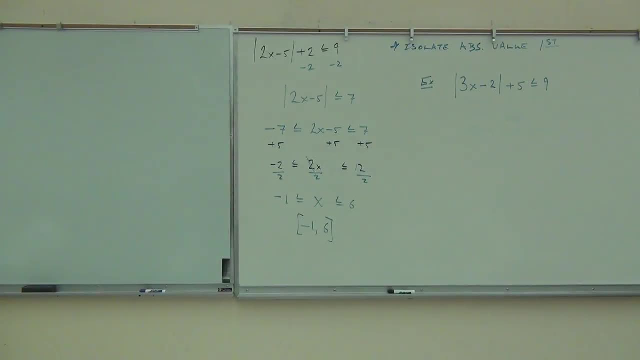 After that, notice that our shortcut is going to work. You've got to notice that part of it. So, first thing, what are you going to do? Good, Did you all subtract that? You didn't go directly to the shortcut, did you? 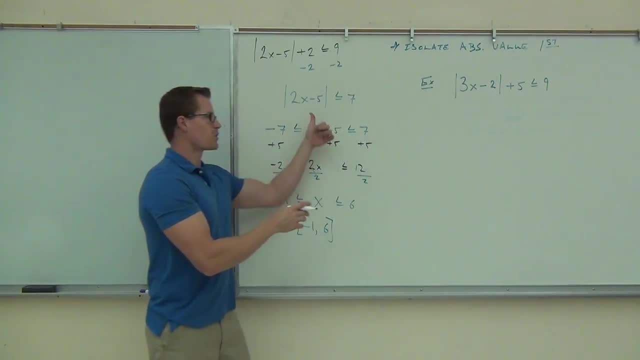 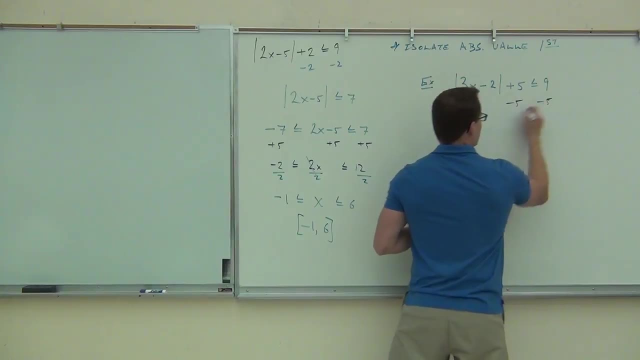 Otherwise the right side. this part would work out fine. This part would work out wrong and you'd get only about a partial credit on that. You don't want to do that. So minus 5, we're going to get the absolute value of 3x minus 2 less than or equal to 4.. 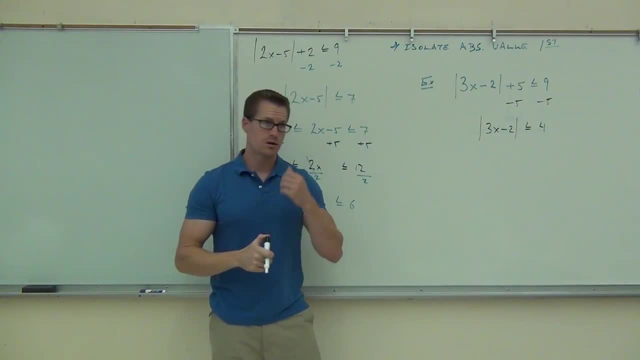 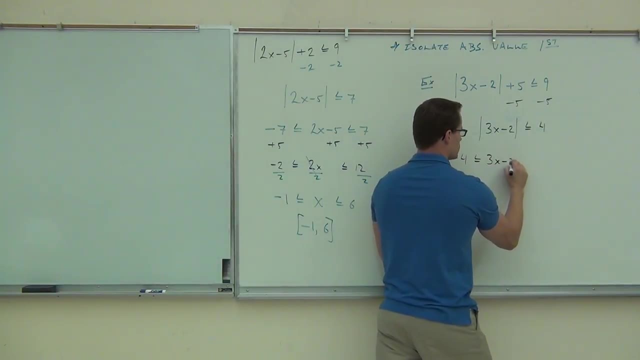 Cool, You all made that far right. Does the shortcut work? Yeah, it's less than, or less than or equal to. That means we're going to take negative 4, less than or equal to 3x minus 2, less than or equal to 4.. 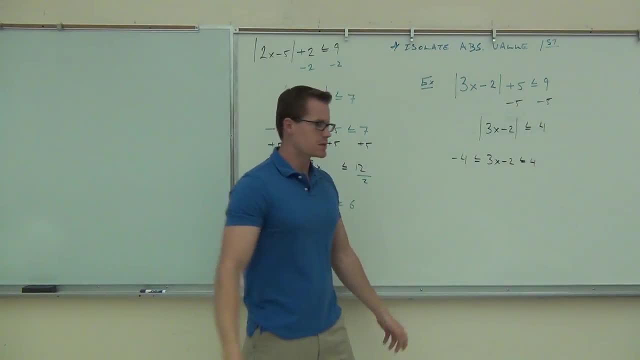 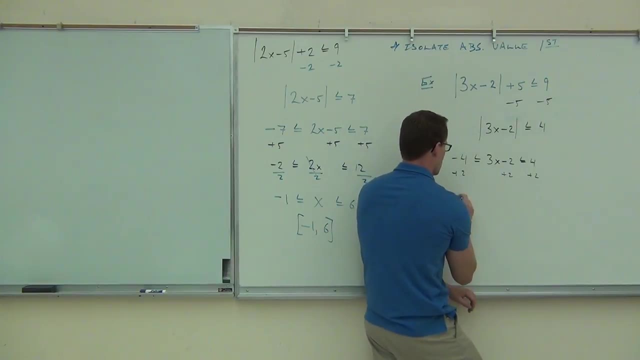 That's a nice shortcut that lets you solve it in just one step. That's great. After this, we're kind of home, Home, free, right. This is the easy part. We're going to add 2.. Negative 2 is less than or equal to 3x less than or equal to 6.. 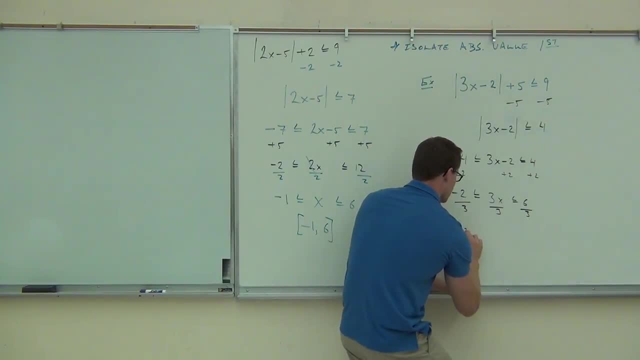 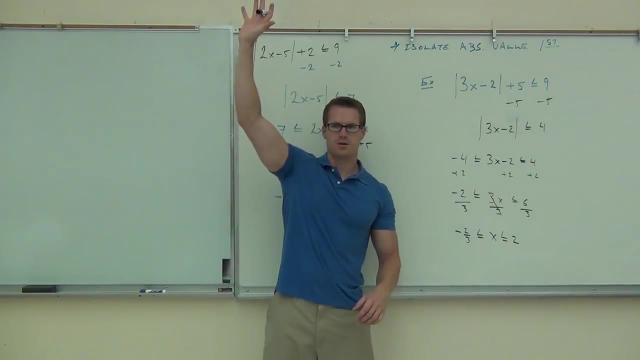 We'll divide everything by 3. I get negative 2 thirds less than or equal to x, less than or equal to 2.. Would you please raise your hand? if you made it that far, Good deal. Can you make it farther? I want to see you all ending with interval notation. 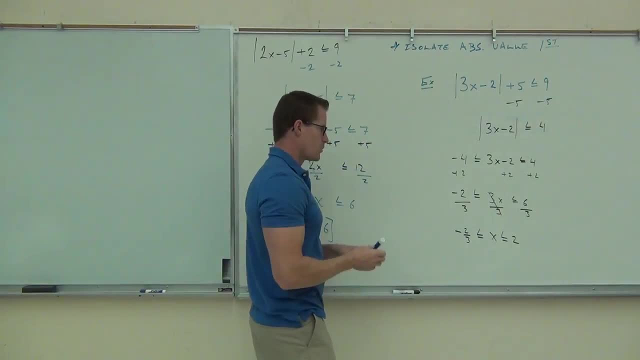 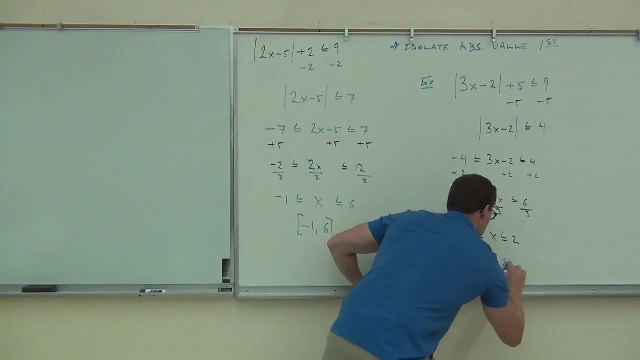 That's what we're going to be doing in this class. So, if we do, where does it start? Yeah, don't let the fraction intimidate you, right? All you have to do is write it down: Rackets And you're done. 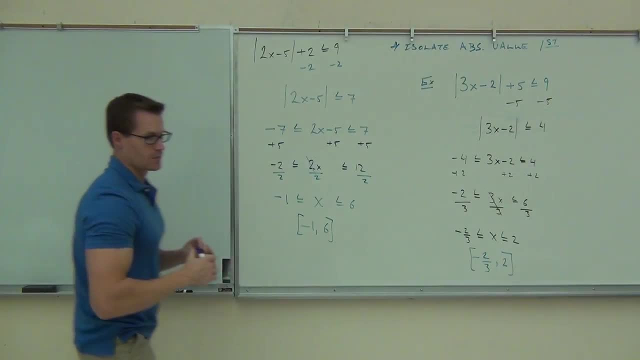 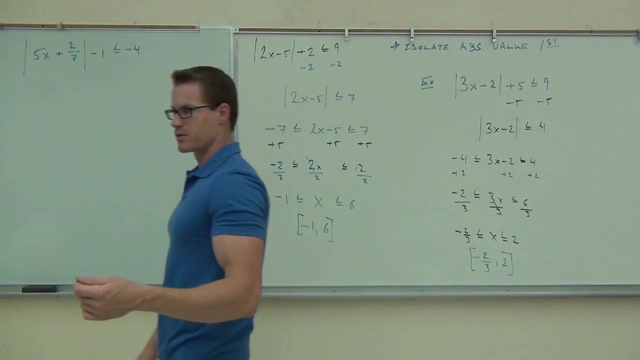 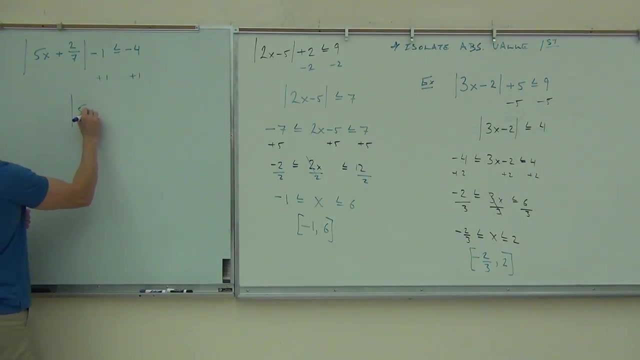 Okay, folks, we should be pros at this. What's the first thing we're going to do on this problem? Add 1.. Okay, so we'll do that. Add 1, add 1.. Absent value of 5x: okay, plus 2 sevenths less than or equal to negative 3.. 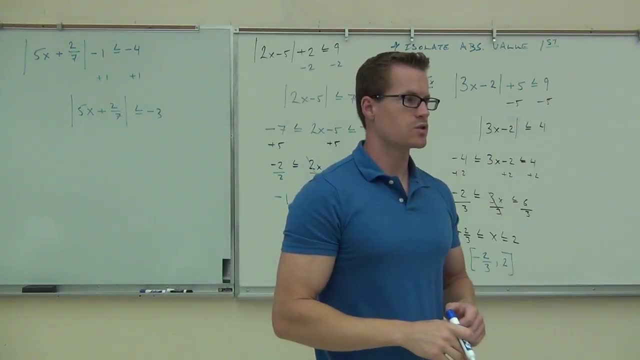 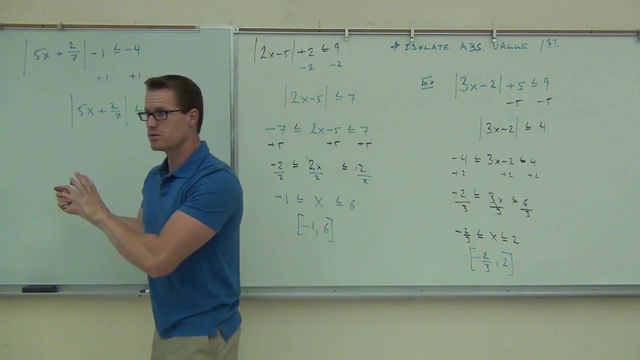 No solution, Solution, no solution, No solution. Why? Because the absolute value is already isolated. Okay, absolute value is isolated, true? Whatever I plug in here, do you agree it's going to be positive? Yeah, Is every positive number in the world ever less than a negative? 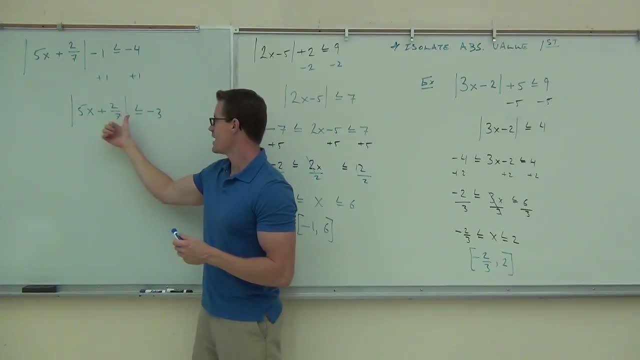 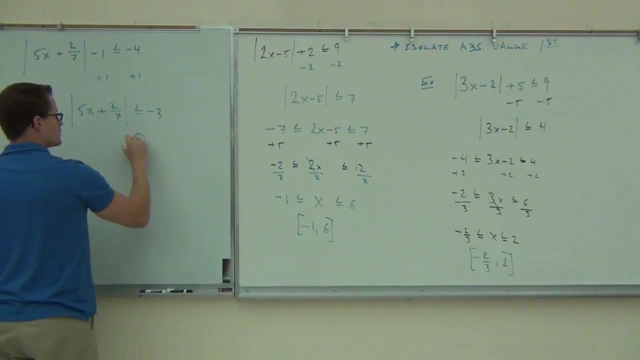 No. Is it ever less than Is? it? Is a positive, ever less than or equal to a negative number? No, This cannot happen, Cannot happen. This would be no solution. That would be no solution. Now let me change the problem on you, okay. 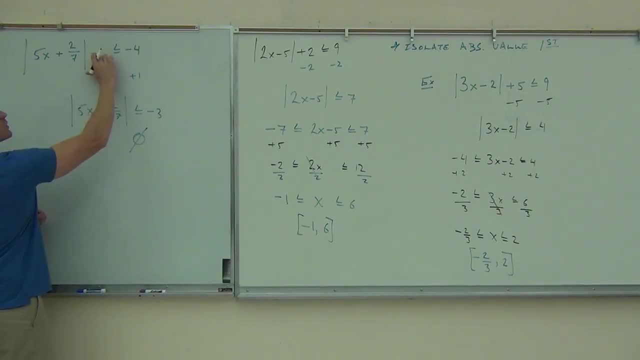 Watch for a second. What if this was no longer minus 1?? This was now minus 6? Would there be a solution in this problem? Yes, Yes, because you add 6 to both sides, This would become a 2.. 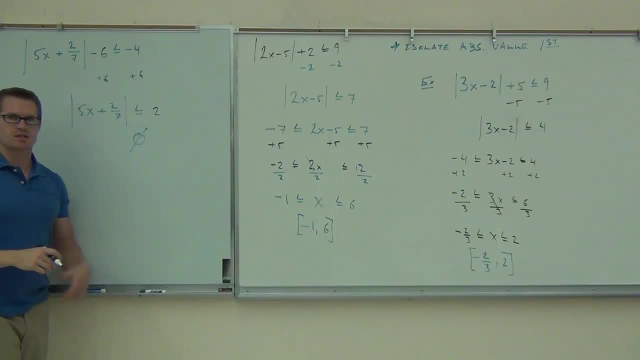 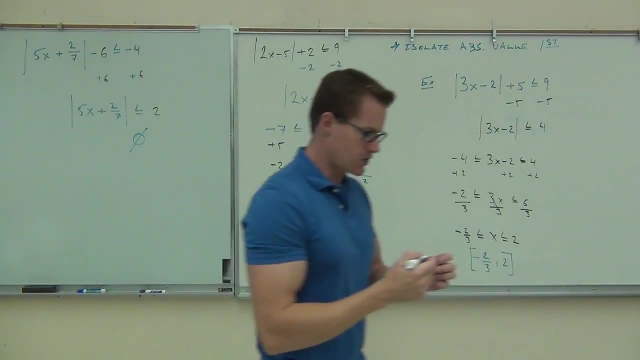 And then you would go ahead and solve that. Do you see the difference on that? So don't just assume because that's a negative. you have no solution. You really have to isolate your absolute value. before you can do that, We're not going to finish that problem. 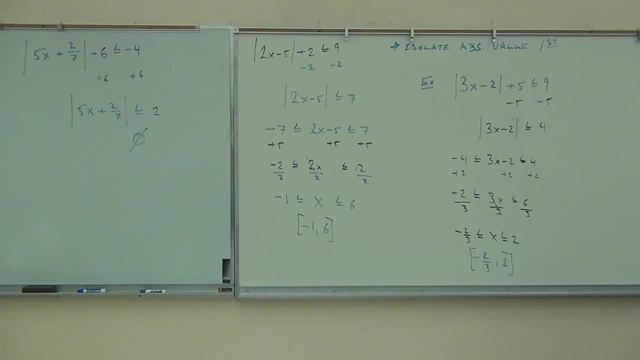 I just wanted to show that to you. How many of you people feel pretty good about that shortcut that I just showed you? Now, of course I told you the shortcut can't work every time. That means there's got to be something else that we can do with these things. 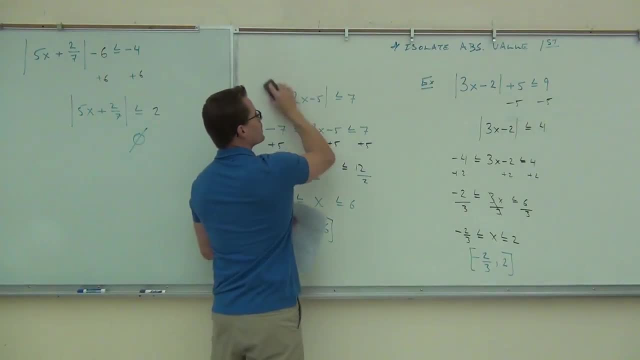 And that comes down to: instead of dealing with a less than or equal to what if I have a greater than or a greater than or equal to What if I have a greater than or a greater than or equal to What if I have a greater than or a greater than or equal to? 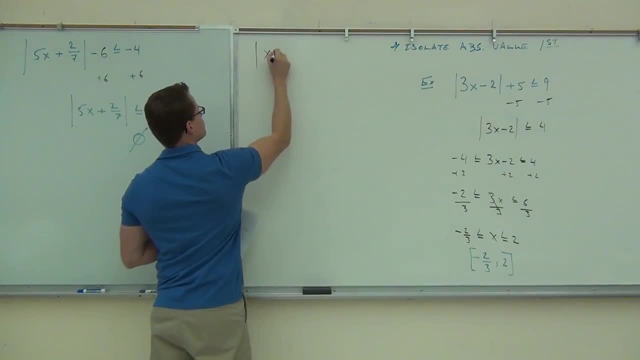 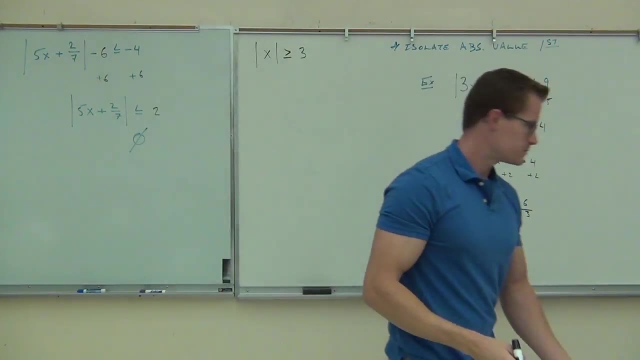 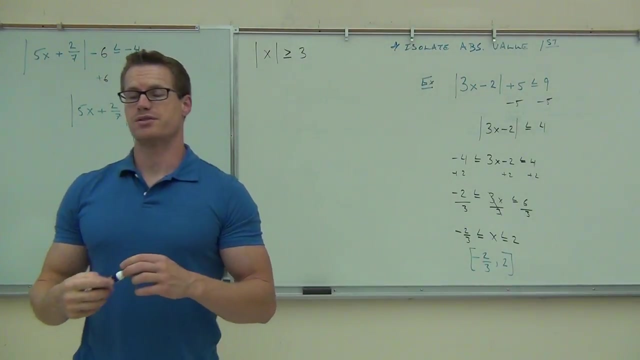 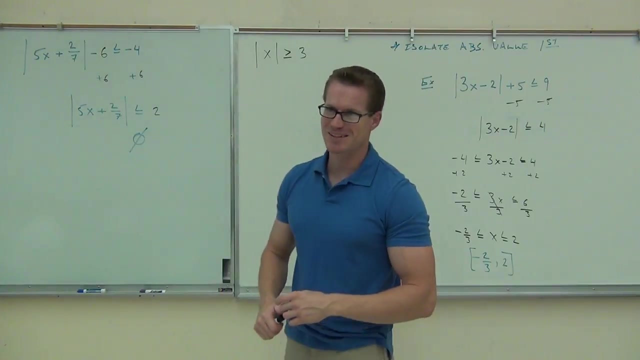 Like this. Now I want you to think of some numbers that are going to work in this thing. Give me one number that's going to work here: Three, Three. okay, Go for the obvious one. That's awesome because it's equal to you. get three. 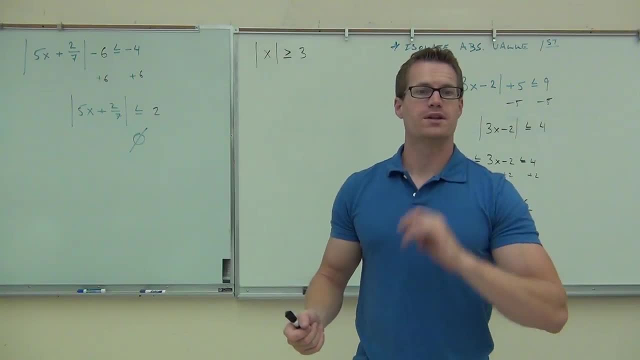 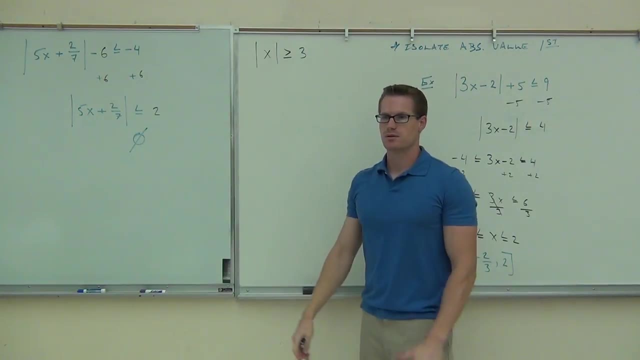 No problems there. What else? Four, Four, let's check four. What's the absolute value of four? Four, Is that bigger than three? Yeah, What else? Infinity, Infinity works. Do you know what infinity is? No, 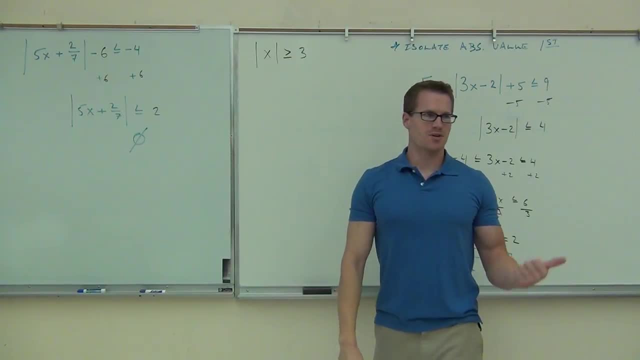 No, I don't either. I wish I did. Four works, five works, six works, seven works, eight works. right, Because all those absolute values can make them bigger. How about negative two? No, Why not? It might have been. 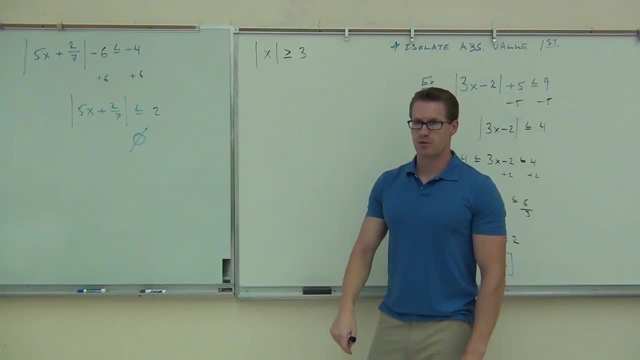 How about two? No. How about zero, No? Negative one: No. Negative three: No. Why negative three? Why negative three? The Ah-ah, yes, that works. How about negative four? Negative five: Yes. 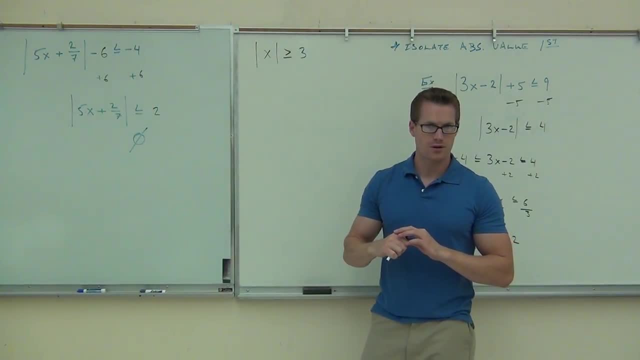 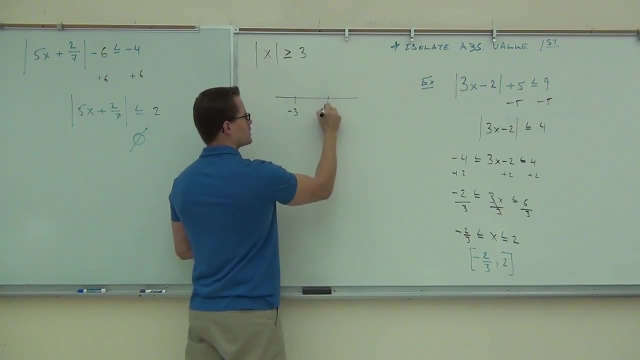 Remember, with a negative number of negative four, what's the absolute value of negative four Four? It changed it positive. So on our graph, here's what you said. You said negative three worked. You said three worked. Do these numbers in here work at all? 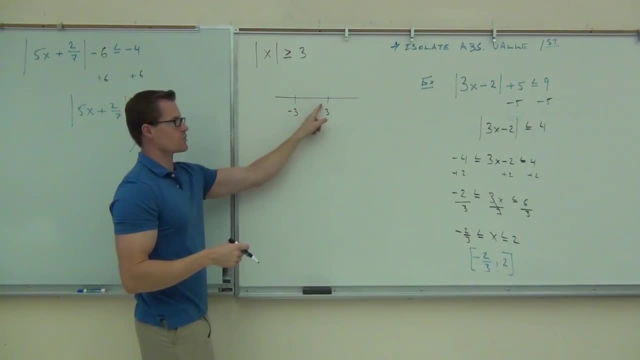 No, We just asked this. Did No, No, None of these work. Did these numbers work? These numbers also work, True. Does that look familiar to you? Remember, This is your or The other one? this is and for sure. 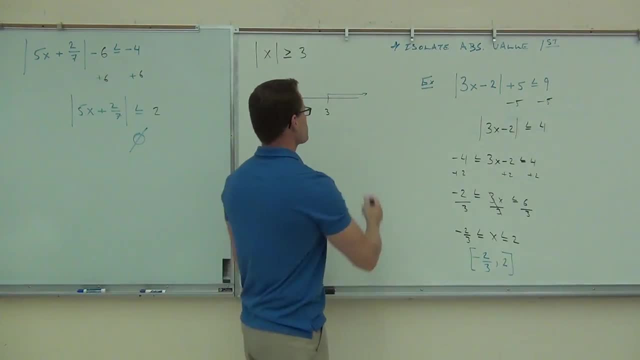 This is your, or That's why we covered both those things. So this is the part where we don't have anything in there. We have this, We have this. This set of numbers or this set of numbers will work. Let's look at an example here. 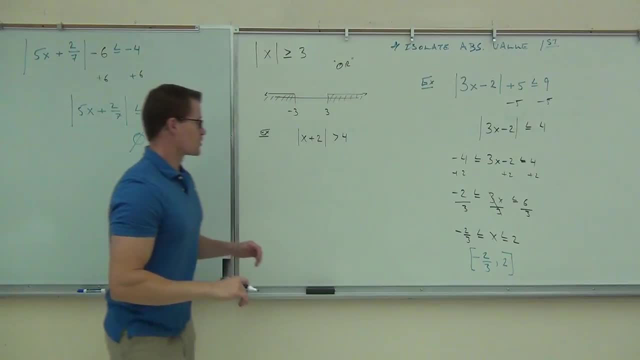 Okay, here's those questions I'm going to ask you again. First thing: is our shortcut going to work on this problem? No, Does it look like this one? No, Heck. no, No way, This is way different. This is not less than or less than or equal to. 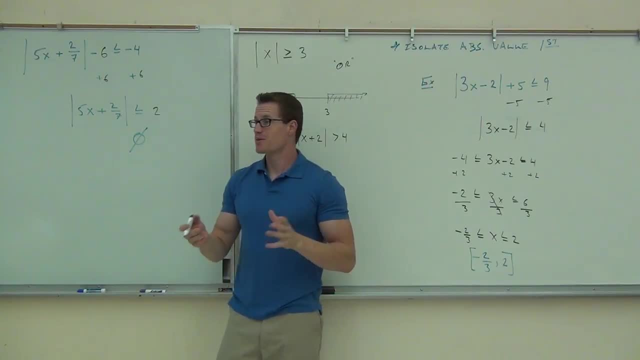 This is greater than or equal to What's actually kind of nice about this? there is no shortcut here. There's no shortcut, And that's kind of nice, because you don't have to manipulate this at all. All you do is you make up your two inequalities and you solve them. 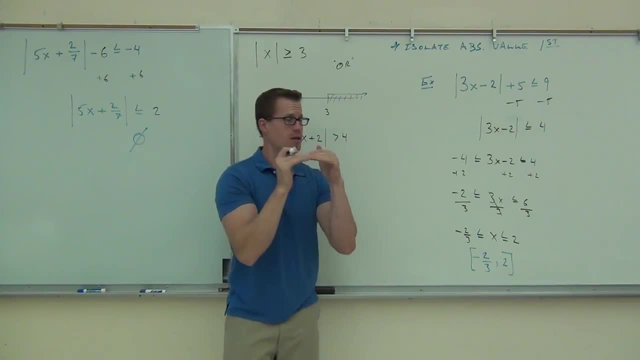 Our shortcut said: we could match things together. right, Because they intersected Here these things. they don't intersect. We can't match them together. Therefore, there's no shortcut. Now do it with me. Shortcut, No shortcut. 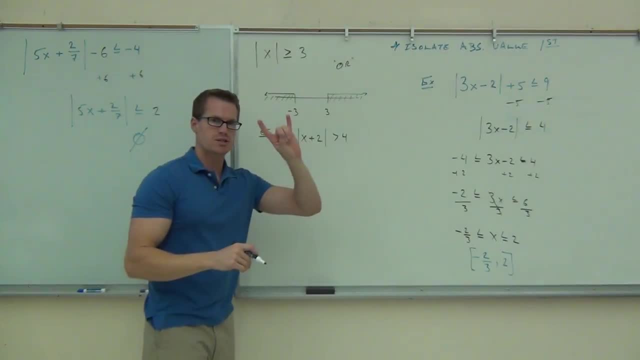 Okay, no shortcut there. So when we do this, we're going to make our two inequalities up, The first one. do we change anything about the first inequality? No, We're just going to essentially drop these signs Again. put this to the right of your paper. 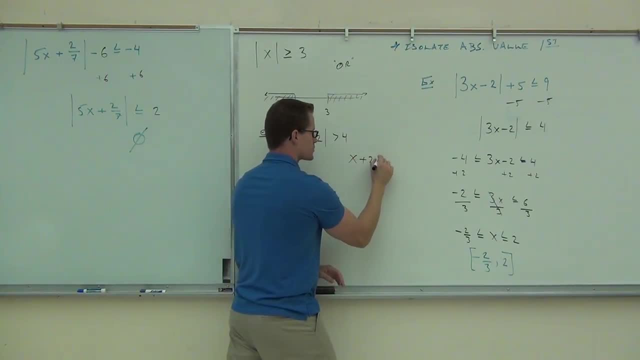 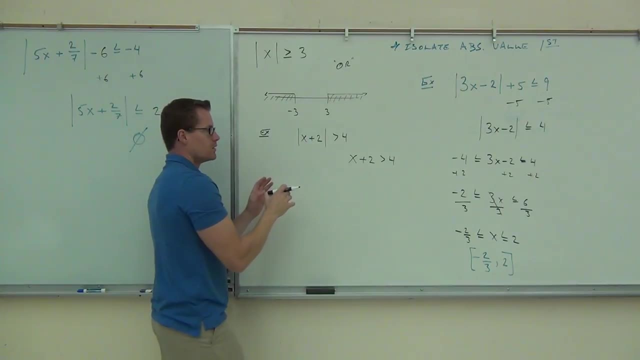 Trust me on this. X plus 2 is greater than 4.. We don't change anything about that. Let's do the other one. What's the other one that I'm talking about? What do we have to write down? We have to put this in. 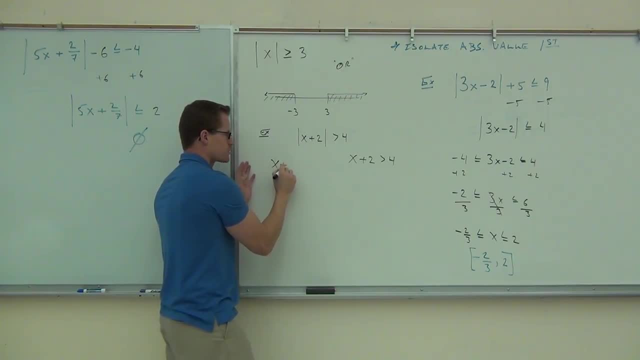 We have to put this in from the initial to the 2nd. Okay, So tell me exactly what I need to write: X plus 2, and then Less than Less than what? Greater than 4.. Perfect, Notice how we're changing the sign of the number and we're flipping the sign. 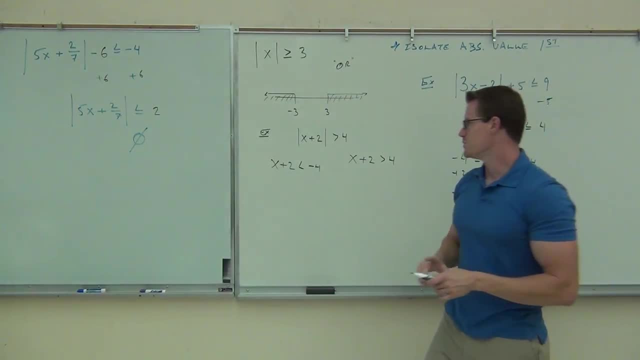 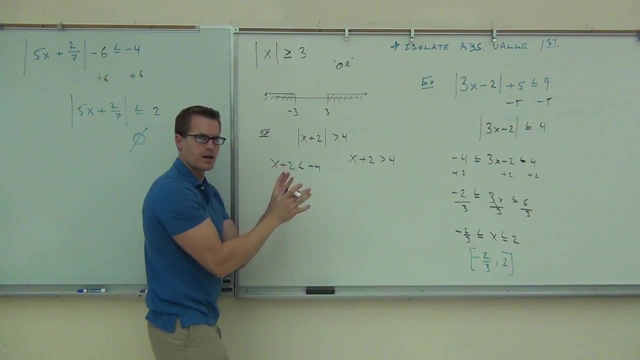 Raise your hand if you're okay with that. Good, That's fantastic. That's exactly what we need to be right now. There is no shortcut. Look how the signs are facing different ways. Even if I reverse them, they'd be facing the wrong way. 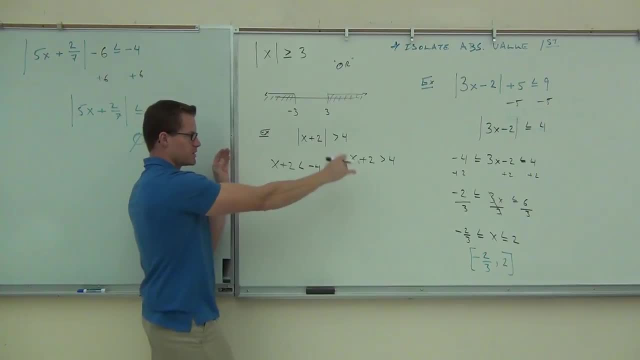 They'd be actually going from a negative to a positive. The signs would be right, but the expression would not be: Okay, It's a. you have a number that's less than a negative and, at the same time, bigger than a positive, and that can't work. 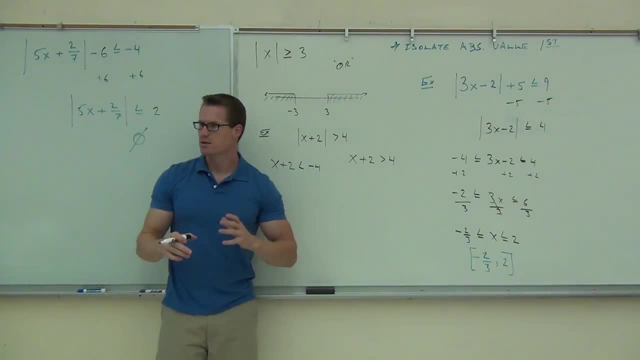 That expression would be meaningless. You cannot do the shortcut with a greater than or a greater than or equal to. Are you with me on that? You cannot do it. All you can do is write your two inequalities. These are talking about an or. 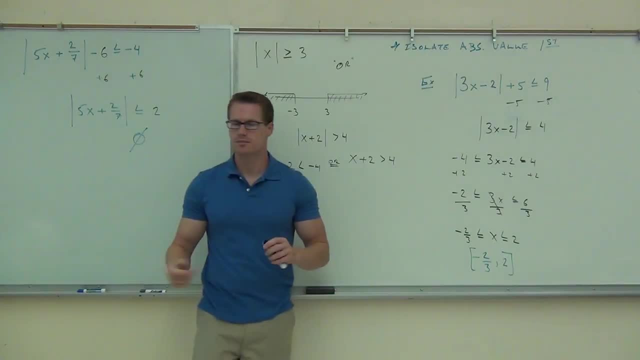 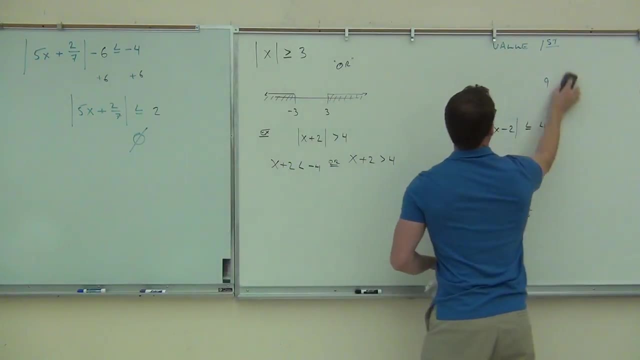 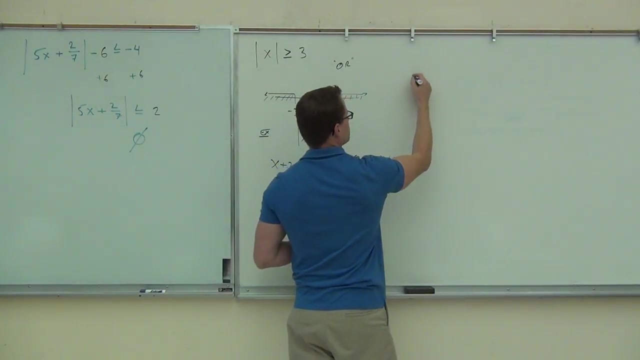 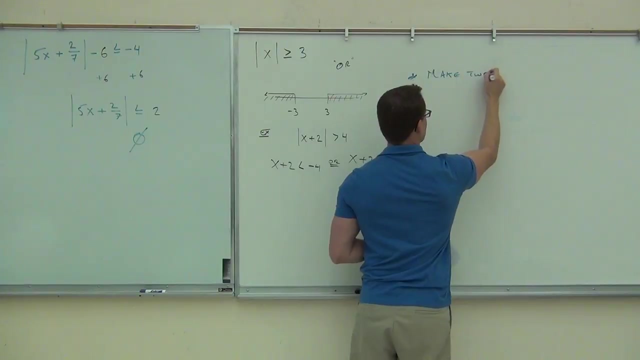 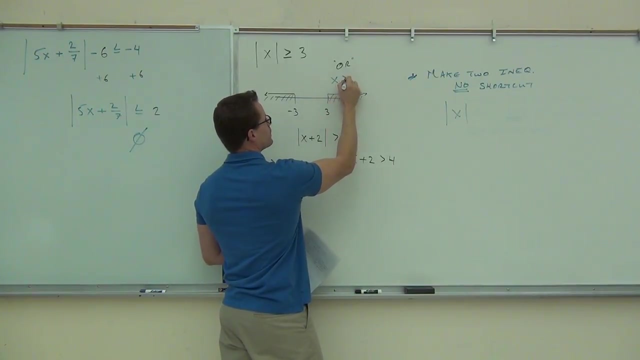 These are or inequalities in the middle, and then solve each one. So what we're doing here: you're still going to make two inequalities, No shortcut. Here's the whole idea. Here's actually what we saw here. What we saw here is that we had x's greater than or equal to 3,. 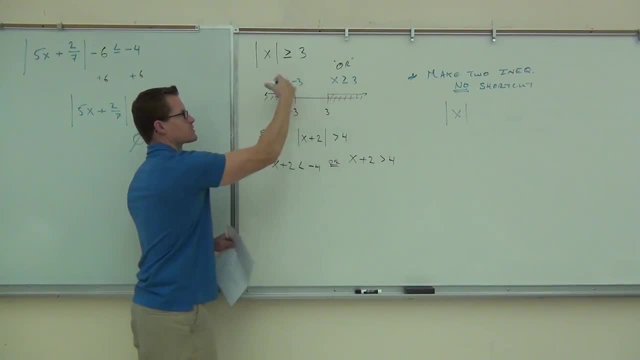 and we had x's less than or equal to negative 3.. That's what we had. We had 1, exactly the same. We had 1 by changing the sign of the number and flipping that sign around. That gave us this graph. 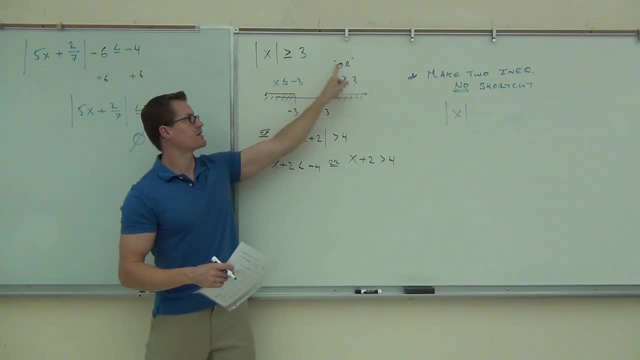 Look at how these graphs match up. Do you see that They do match? 1 is exactly the same 1,. I changed the sign and flipped my inequality, and it gave us this portion of our graph. That's why we have to do that. 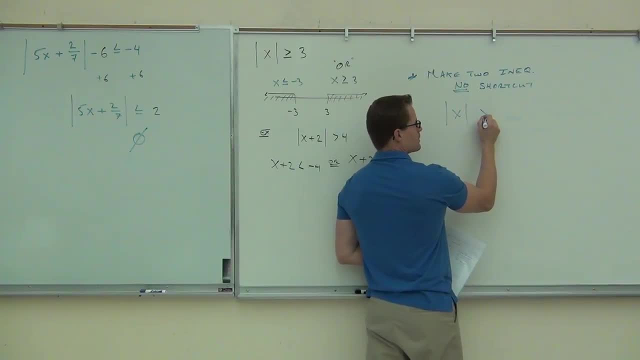 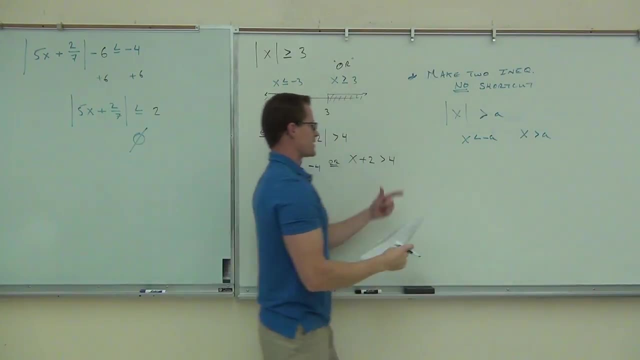 So, for any absolute value of x is greater than, or greater than or equal to a, we're going to do: x is greater than a, x is less than negative a, and that's what we're doing in our case, right here, And we're going to solve each one. 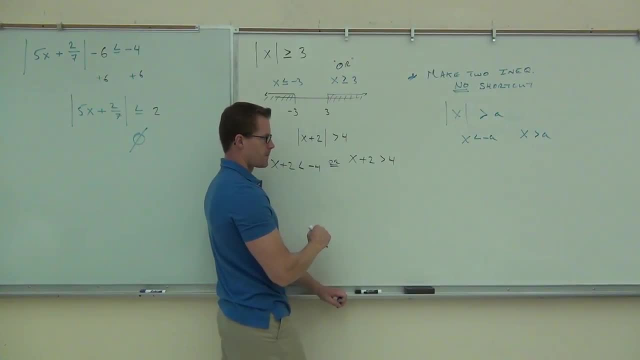 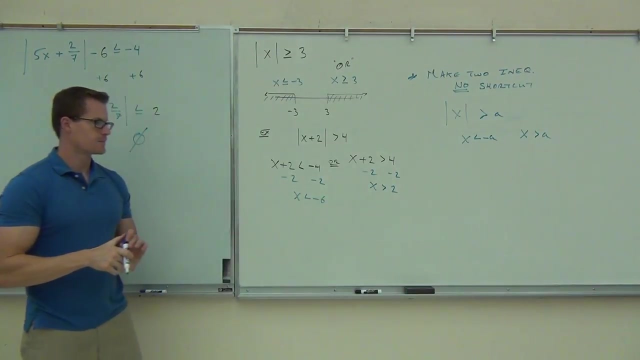 So let's solve this. How do you solve the right one? x is greater than 2.. How about this one? x is less than negative 6.. So far, so good. Hey, here's why, by the way, I had you write the first one on the right-hand side. 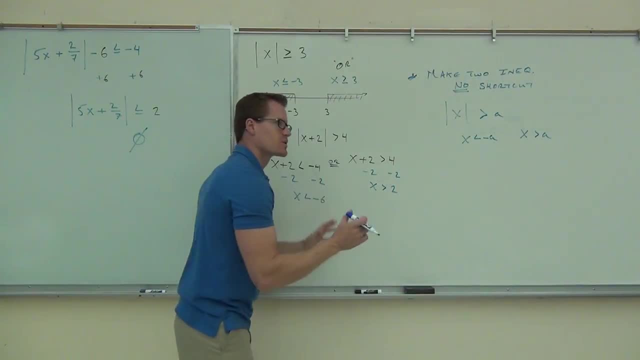 Because if you do that, check it out, Most times, 95% of the time when you do your number line, it's now in order. See how it's in order now. You don't have to switch things around. That makes it kind of nice, right. 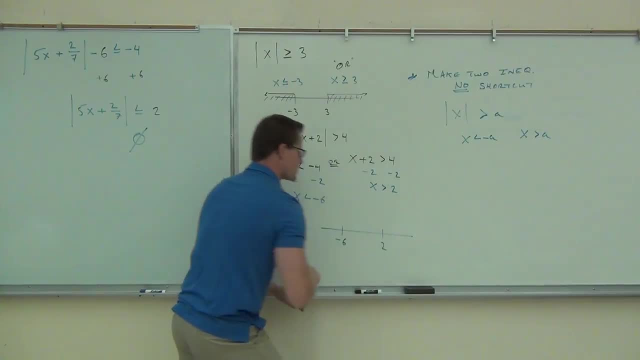 So we're going to have our negative 6,, our positive 2.. It's already in order. Guess what This is? an or inequality, right, Or 99% of the time, 95% of the time, it goes like this: 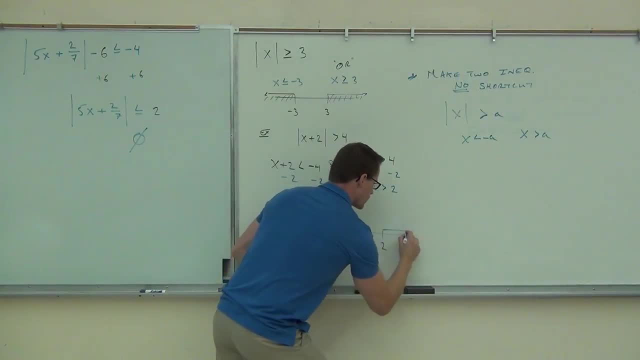 That's what it does. So if we have x bigger than 2, we know we're going that way. If we have x less than or equal to negative 6, we're going that way. We've done this a lot. 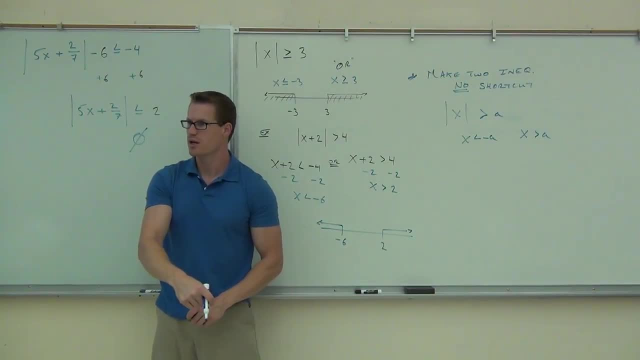 That's why I'm kind of going quickly through it. We should have mastered this concept at this point. Can you do your interval notation from here? Where does this interval start? Negative, Negative To where Negative: 6. Good Parentheses. 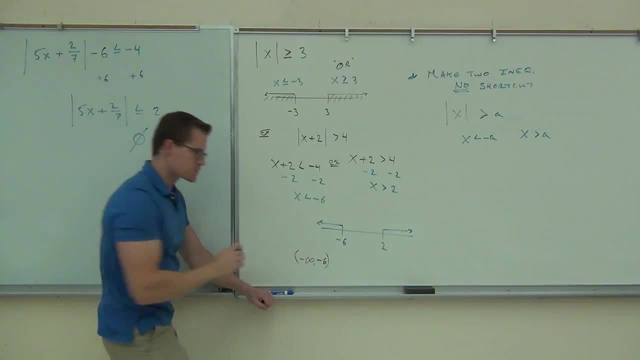 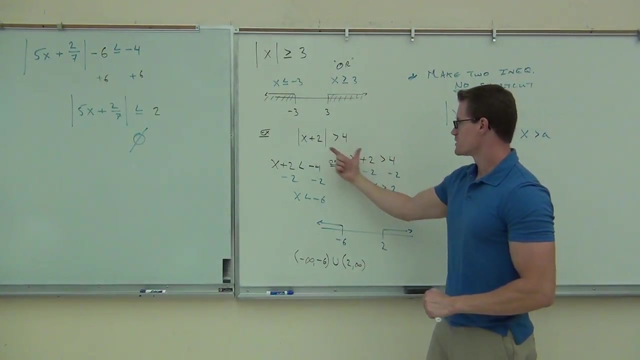 Parentheses: What goes in the middle of our two values, Two segments? here We go: 2 to infinity. So here's our idea. Idea is make your two inequalities, one positive, one negative, with the sign of the second one. 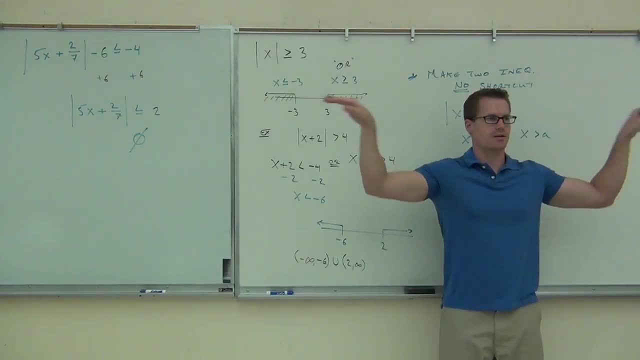 Then inequality of the second one. Solve both of them down. Chances are you're going to get math. That's most likely what's going to happen. Let's try a few more. I'll give you one to do on your own, as I'm erasing some stuff over there. 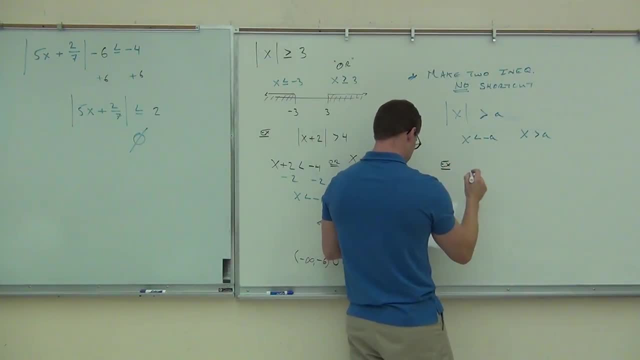 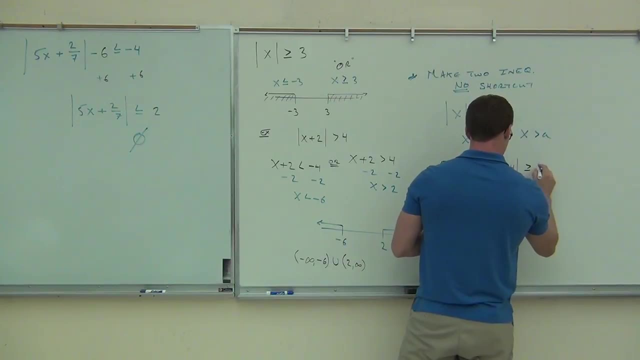 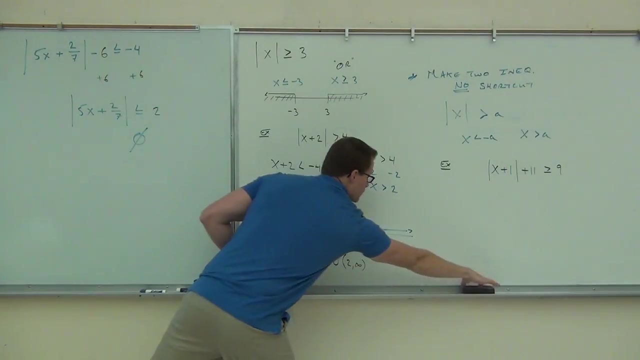 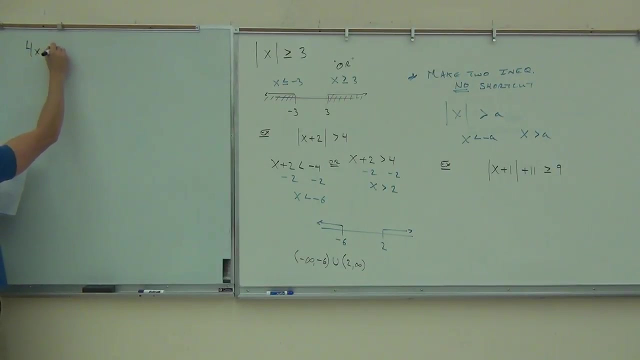 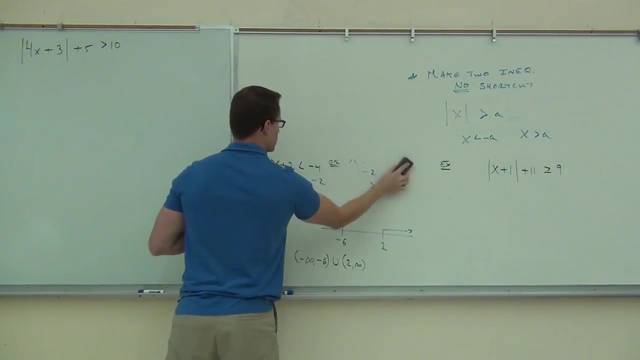 And then we'll call it a day. There you go, So work on that one. If you finish that one and you're feeling pretty good about it, try this one. We'll take about one more minute to see if we can wrap up that problem. 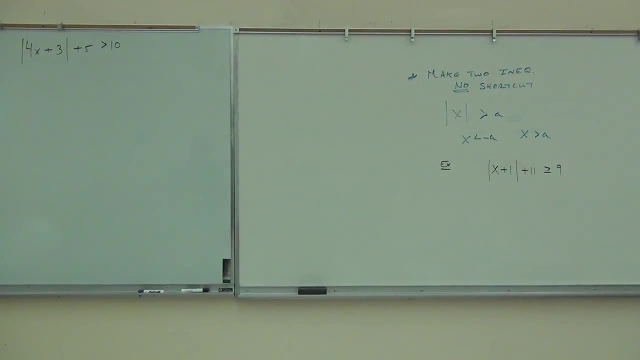 If you finish that one, first, do the second one. Okay, let's work on the first one together. Hey, does a shortcut work for this problem? Did you all shake your head? Should I be asking about the shortcut yet What's the first thing you should be doing? 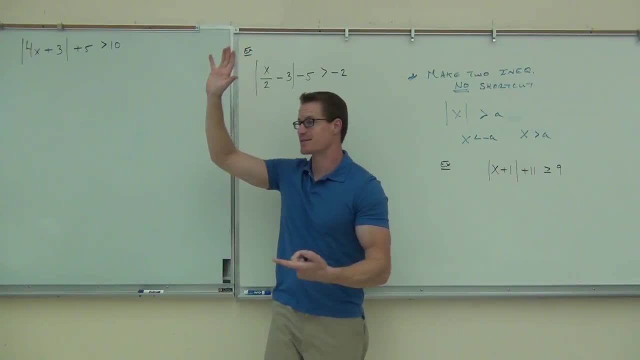 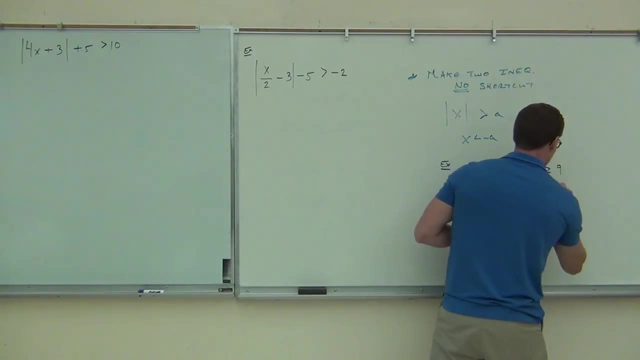 Track 11.. Track 11.. Oh, we'll subtract 11 right off the bat. Good, That's fantastic. You need to be doing that. So subtracting 11.. Greater than or equal to how much Negative 2.. 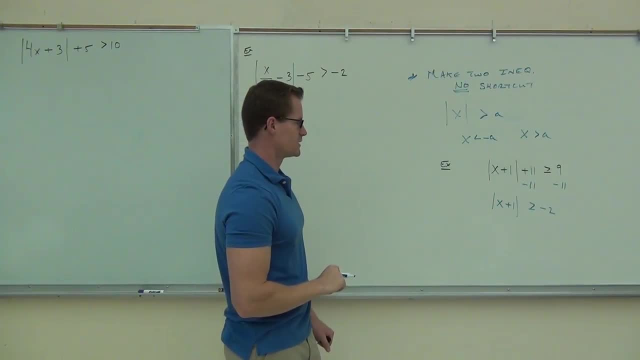 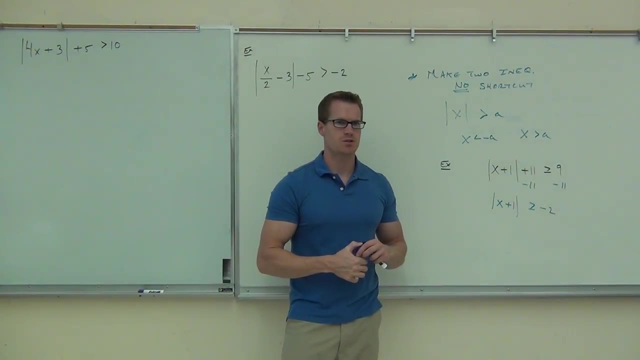 Whoa, That's weird. What do we have here? Numerous solutions, Numerous solutions. I want you to think about it For a second. I want you to think about it For a second. Think about it for a second. What's absent value do? 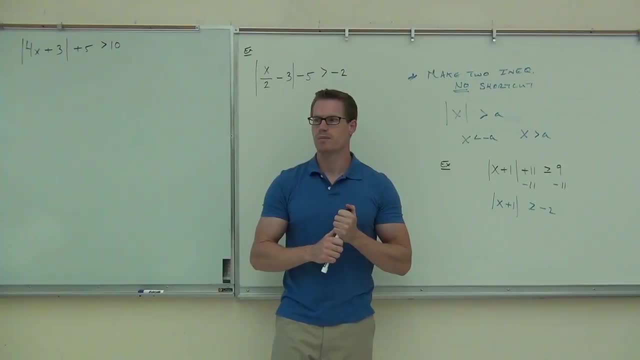 No matter what makes positive right, No matter what, No matter what it makes a number positive. Is a positive number ever bigger than a negative number? Is a positive number always bigger than a negative number? Yes, You agree, that's a positive number. 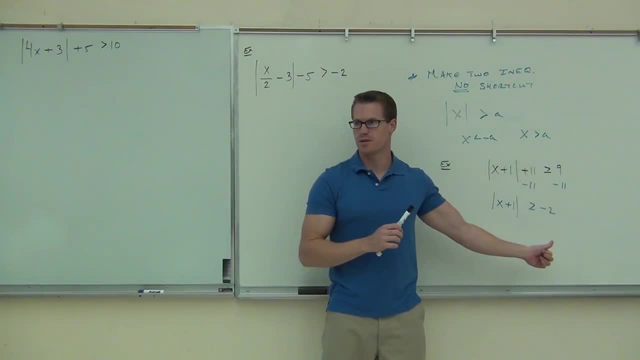 Yes, negative number right, Always, Always bigger than the negative number. This is all solutions. This is infinite solutions. Negative infinity to infinity. This is one of those ones where your or would cross over. right, You can't solve this. It doesn't make sense to actually. 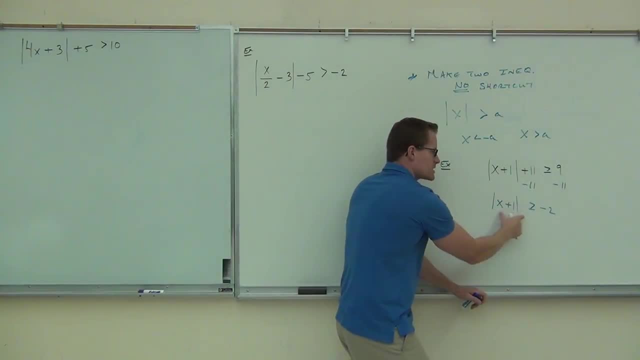 write out the inequality. But if you have a positive greater than a negative, that's true all the time, No matter what you plug in. Try any number. okay, Give me just some crazy number. One's a crazy number, Crazy. How about negative 53?? Add one to negative. 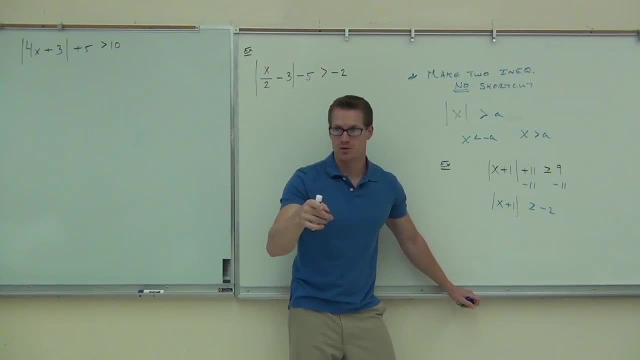 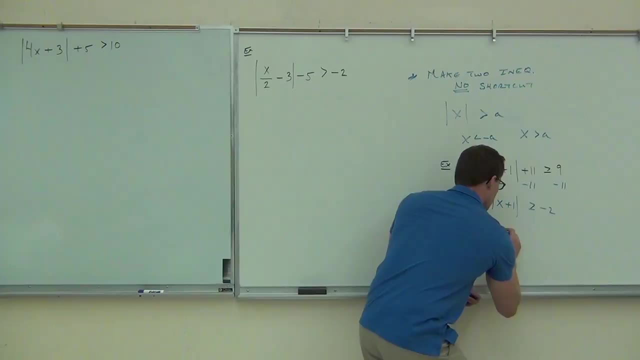 53. What do you get? Negative 52. Take the absolute value of negative 52. What do you get? 52. Do you see how, when you take the absolute values, you become positive? Is that greater than negative 2?? All the time, No matter what you plug in, And that's what this. 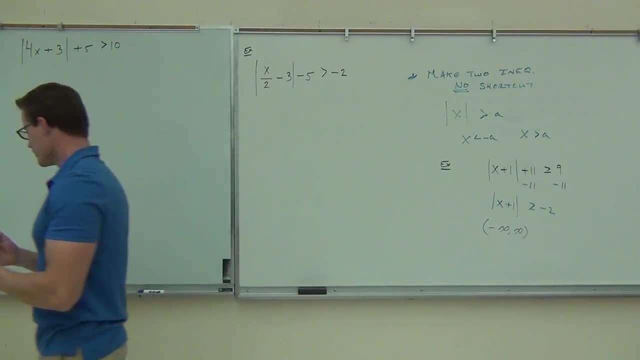 says: No matter what I plug in, that's always true. Okay, now we can try this one. all right, Let's all work on this one together. What's the first thing we do on this problem? Sorry, I kind of threw a curveball at you on that. 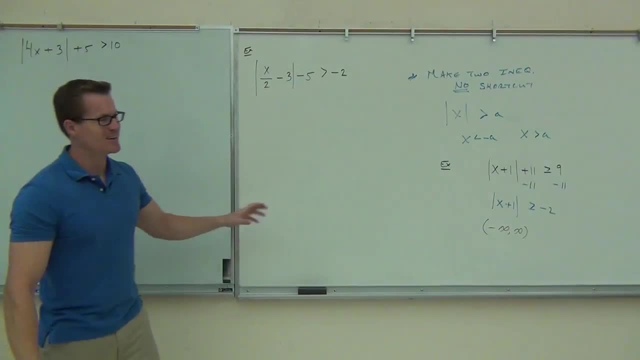 one. You're like wait a second, Leonard, This is too easy, No solution? Well, I think it's all solutions. How about this one? What do we do here? Let's all work on this together. If you participate up here, we get. the absolute value of 4x plus 3 is greater than 5.. You? 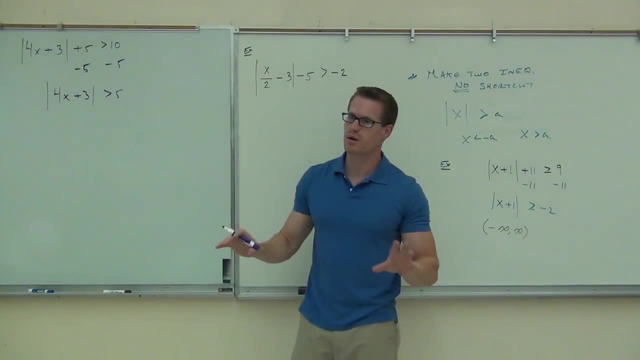 all need to isolate the absolute value first. That's the first thing you do, And that's the first thing you do, And that's the first thing you do, And that's the first thing you do. you all come up from here 3 times. Okay, we'll do that. 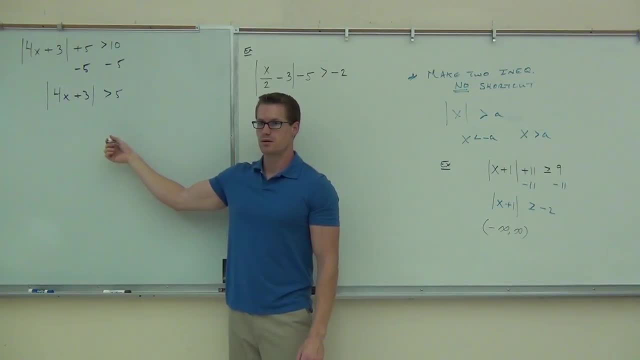 Okay, No way. What should I do? I should have been more stringent than I am. No, No way. No, running on it In thebecause I think there is actually a change in your logic. Is it going to be greater than or less than? 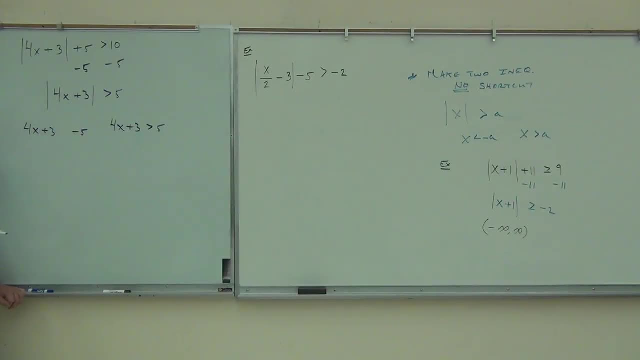 Less than. I'm hearing both people. I'm hearing people say Less than Less than. We have to switch that around. We have to switch it. You change the sign. you flip the inequality Folks on this type of inequality. look at your symbols here. 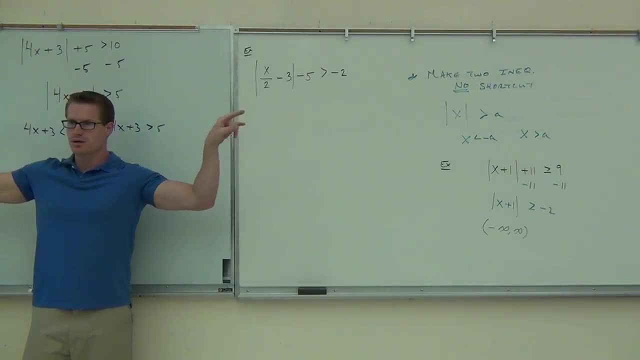 They will be facing different ways. They're going to be facing the wrong ways. Well, the correct ways, but different ways, not the same way. Subtract 3. We get: 4x is greater than 2. Divide by 4.. 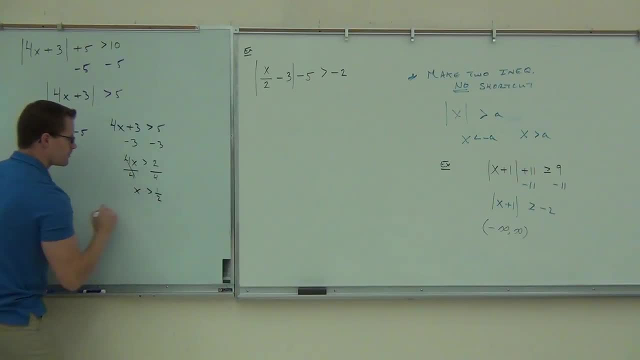 Don't change anything around. Greater than 1 half Subtract 3.. 4x is less than negative 8. Divide by 4. x is less than negative 2.. Can you graph this on a number line? Yes, Do that. 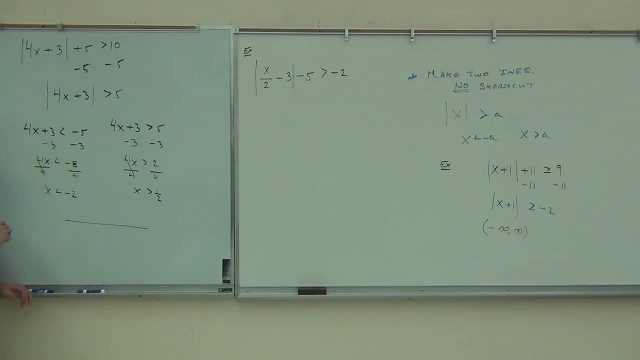 Let's do that together. Where does it start? Negative 2.. Notice, if you do this in the correct order, it's already there for you. Negative 2, 1 half. Let's do this one first. Folks, should we go up and to the left or up and to the right here? 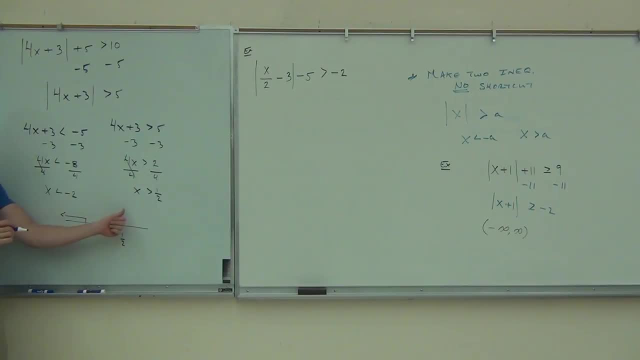 Up and to the left, And on this one do we go up and to the left and up and to the right? Which one Right? Can you graph this with an interval notation or do interval notation with that? Yes, Negative 2.. 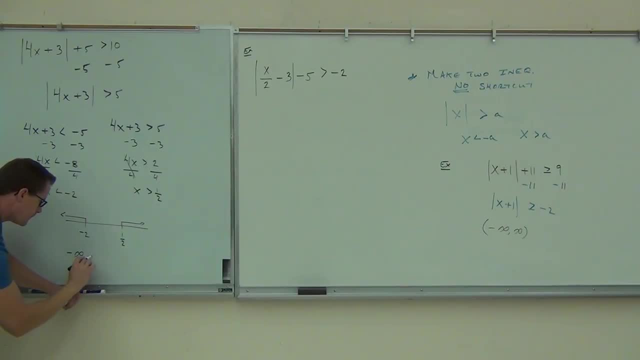 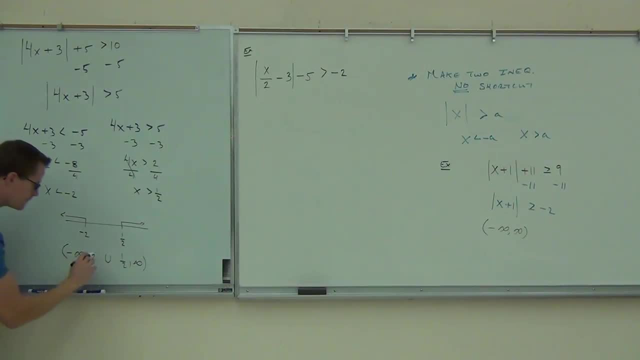 Parentheses, Parentheses. As good as we can do, I want to show a hand, somebody to be able to get. with that example, Yes, How about this one? What are you going to do? first, Add 5.. Add 5.. 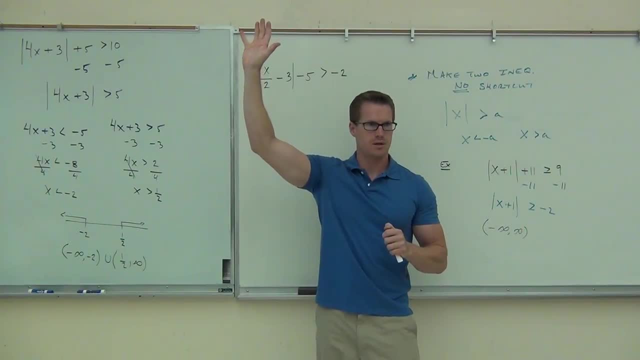 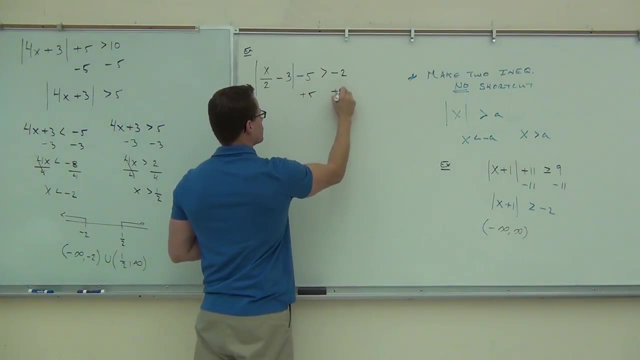 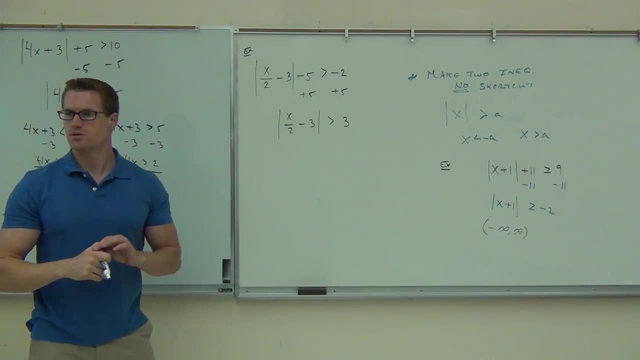 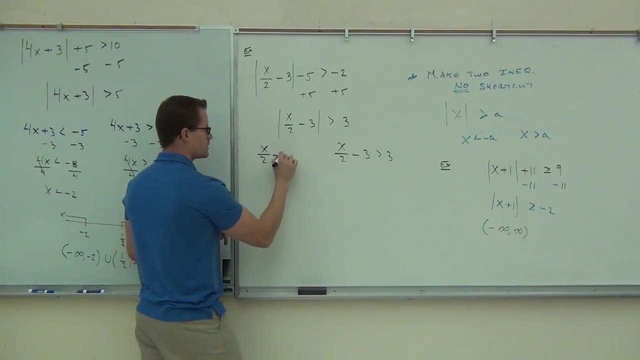 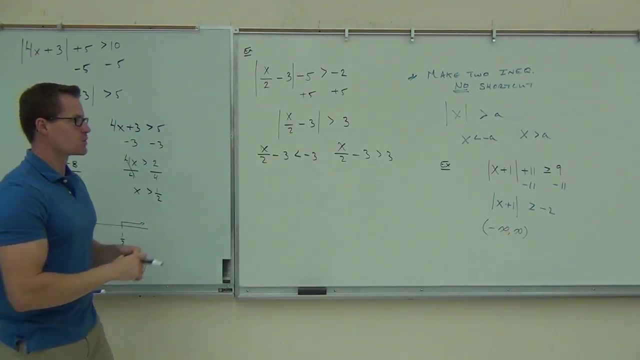 What now? Two inequalities: First one we do without changing anything. Second one we do by changing the sign and the inequality. It's this part, right there. That's the important part. I just want to make sure you don't get stuck on these fractions again. 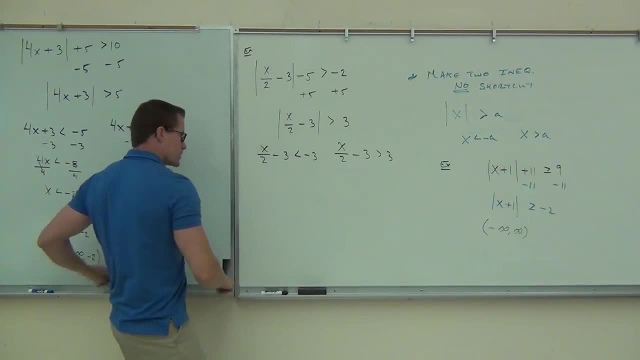 Some people kind of make some mistakes in their homework with this stuff. When you're doing this, try adding the 3 first. okay, And get x over 2.. In this case, it's less than 0.. x over 2 is greater than 6.. 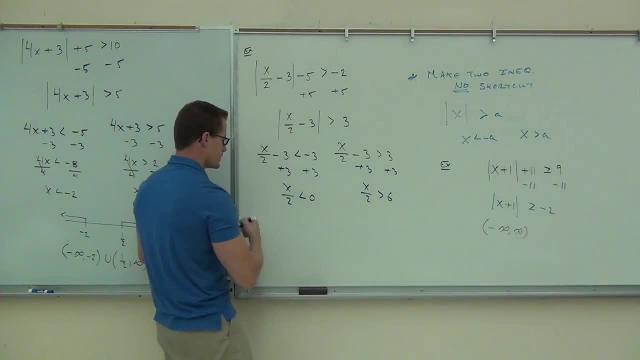 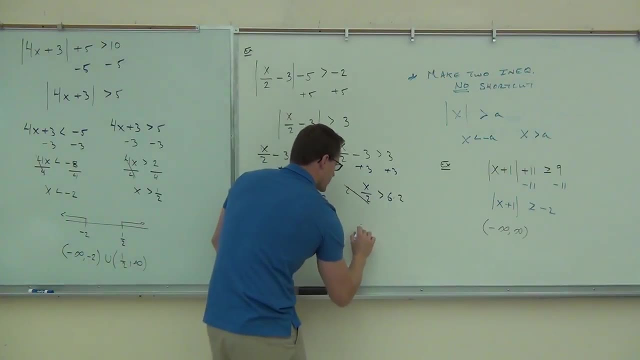 Now multiply by 2.. That way you don't make any mistakes on that. If we do, we get x is less than 0.. We get x is greater than 12 with our- I'm not going to do the number line. 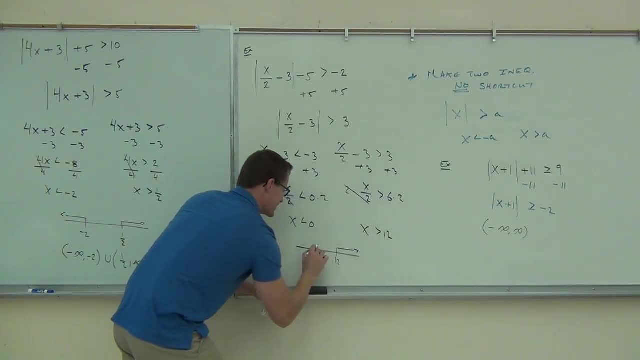 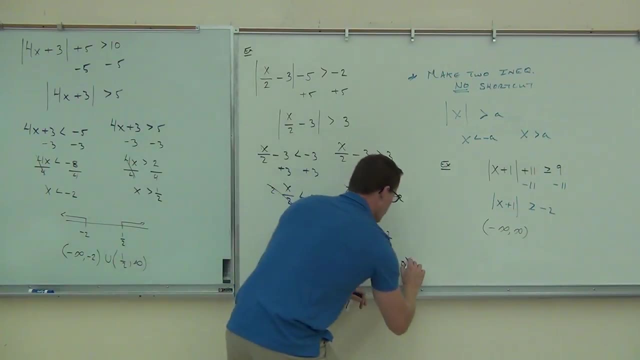 Well, I can say: well, here's 0 and 12.. It's so fast, It doesn't really matter. Negative infinity to the 0.. We use some parentheses there because we don't have an equal sign. Union 12 to infinity.